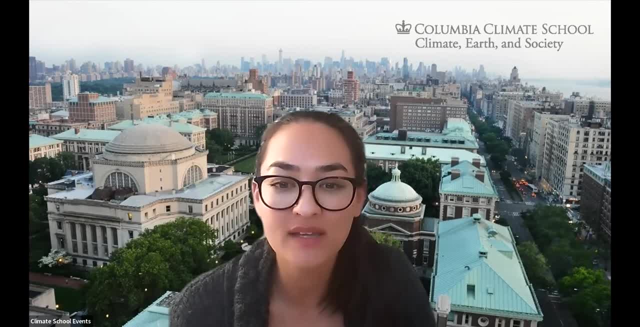 centers and over 700 people who collaborate among different departments at the university so we can better connect, amplify and advance new areas of climate research, inquiry and impact across Columbia and beyond. So what we're hoping to do with these Climate Live K-12 sessions is 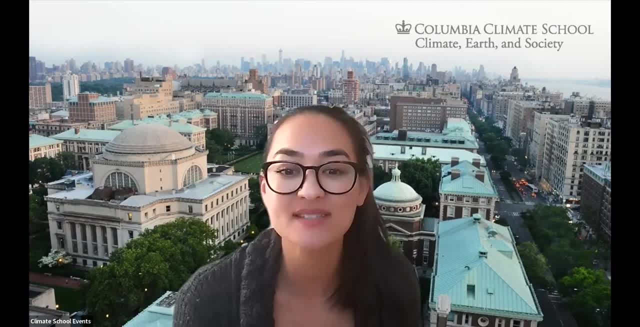 to share with you the interdisciplinary work through our scientific experts. These are monthly sessions that we've run throughout the academic year, so for the 2022-2023 year, we're going to run through the month of June. If you'd like any more information about the sessions that we've, 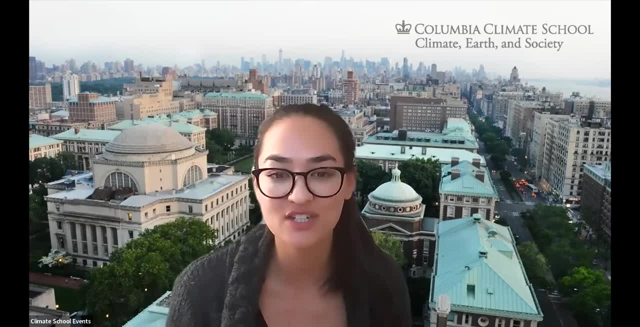 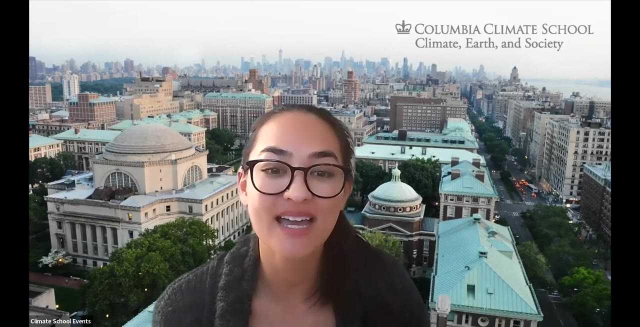 already ran or future sessions. you can visit our website that I'll put in the chat in just a moment, or you can contact us directly via email. Each week we focus on a particular topic, and each topic is tailored towards a certain age range. So for today, the session is titled The Climate Symphony. 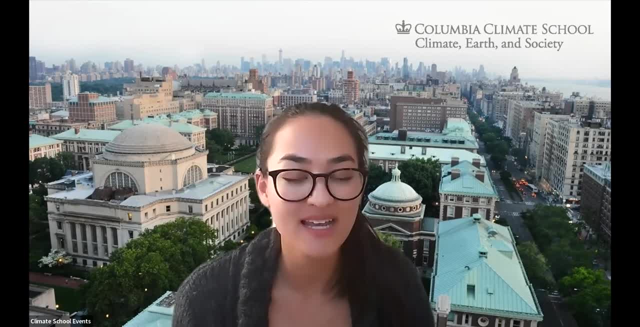 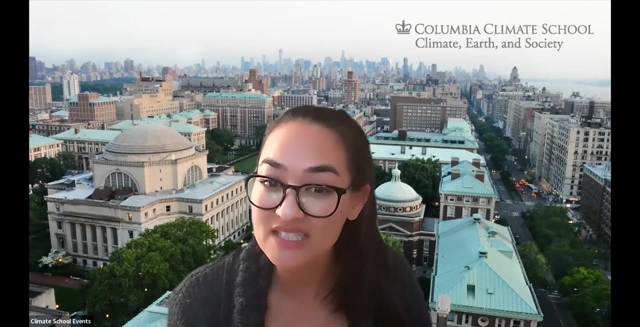 How Climate Variability Impacts Global Rainfall Patterns. So climate variability plays an important role in our system, and it impacts rainfall differently from year to year and from decade to decade. This presentation will focus on different modes of climate variability and their impact on rainfall, the difference between climate variability and climate change, and what 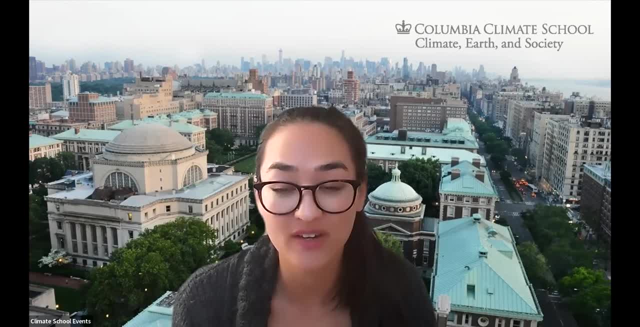 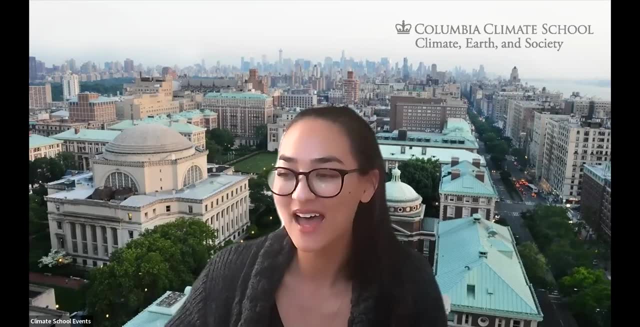 happens when different modes of climate variability impact on rainfall. So let's get started. So the goal of this session is to really think of the climate system as an orchestra playing a symphony, And so today we're joined by Laurel DeSera, who will be leading us in this session. 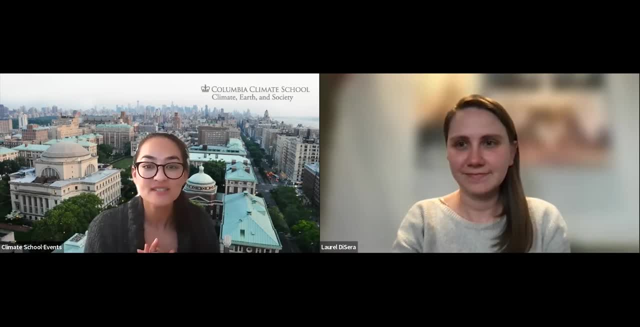 Just a few logistics about Climate Live, So we have time for questions halfway through the presentation and also at the end of the presentation. We encourage you to use the Q&A box so we can monitor those questions and ensure that they get answered, And usually we have. 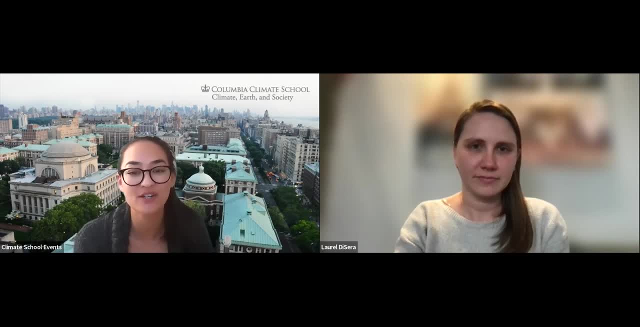 the chat box disabled, but for this special session we really want to hear from you all, So the chat is enabled. Please use the chat to answer the questions that Laurel asks. And just so everyone knows, this session is recorded and we can send participants links. 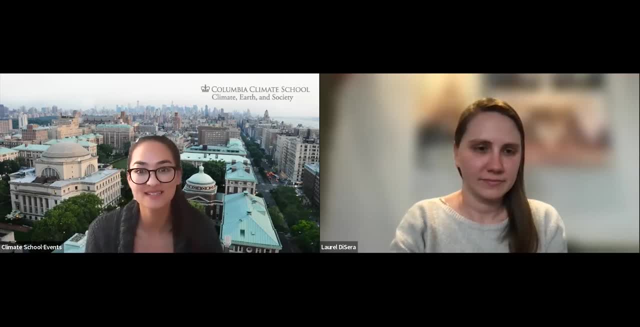 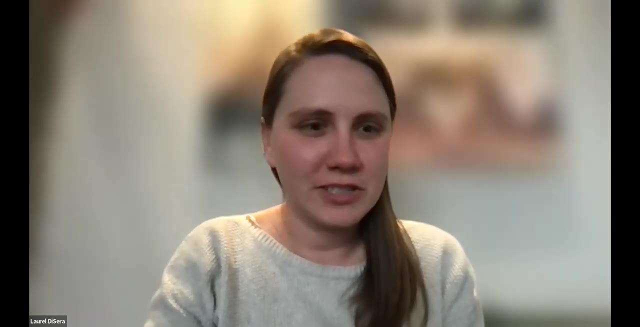 to this recording after the end of today's Climate Live. So, without further ado, I will pass it over to Laurel DeSera. Good afternoon Everyone. Hopefully you can hear me and it all looks good. I'm just going to share my screen now. 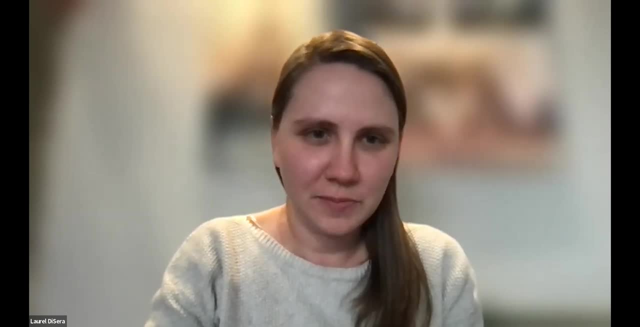 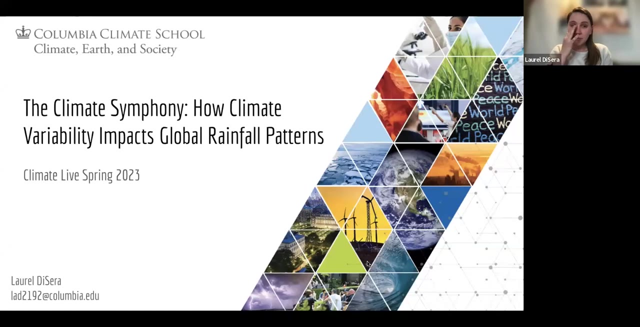 So we are all on the same page. Hopefully you're going to get it. There we go. Hopefully, let me know if you can't see, But my name is, as Laurel mentioned, my name is also Laurel. I am a current PhD student at 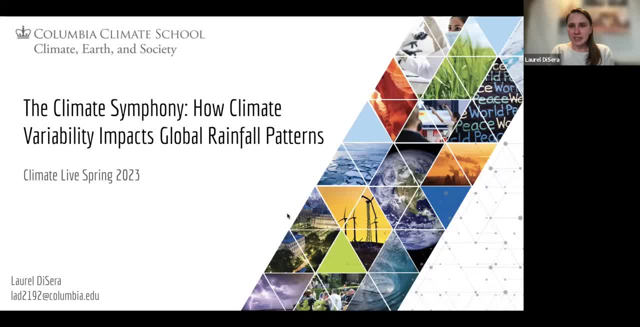 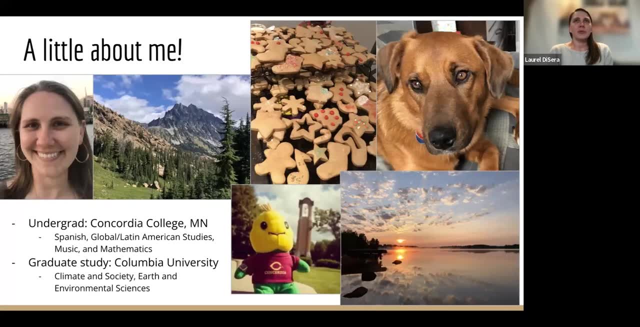 Columbia University And we're going to be talking about the Climate Symphony today. A little bit about myself, So I'm a pretty non-traditional climate scientist. I did not study physics in my undergraduate degree. I was very interested in the math and sciences. However, I had interest in a lot of 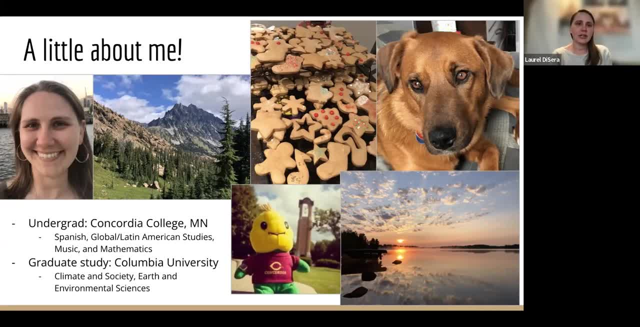 different areas. So I finished high school in Minnesota and I then went to a smaller liberal arts undergraduate college called Concordia College in northern Minnesota, which was a pretty close to the Canadian border, so pretty cold up there, Don't you know? you know the little. 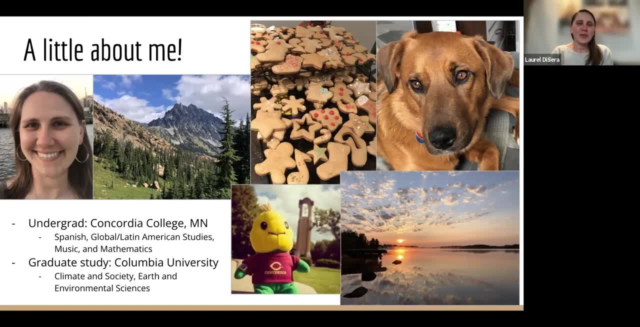 Minnesota accents that people are familiar with, And our mascot was actually a corncob. So you know that's pretty much everything that northern Minnesota is is just growing corn. However, I was really interested in a lot of things. Like I mentioned, I was interested in Spanish global. 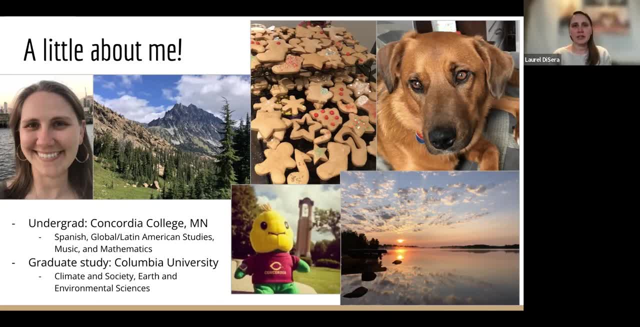 Latin American studies, music and mathematics. So this kind of shaped my time during my undergraduate And I was actually really lucky to be able to study abroad during my undergraduate career And I studied abroad in Argentina And while I was there the country experienced really dramatic impacts. 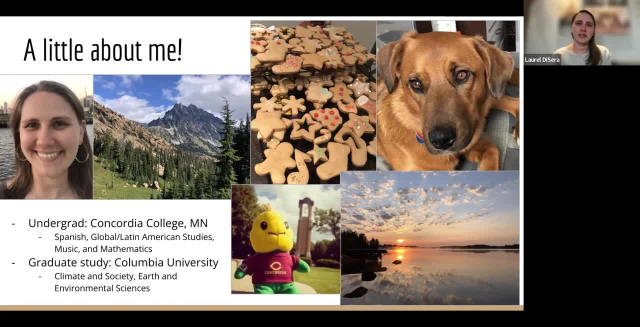 of rainfall, And that's what really got me interested in studying climate science. So after my degree in undergraduate I worked for a couple of years at a nonprofit and then went to study here at Columbia University for my master's, where I did the master's in climate and society, And then 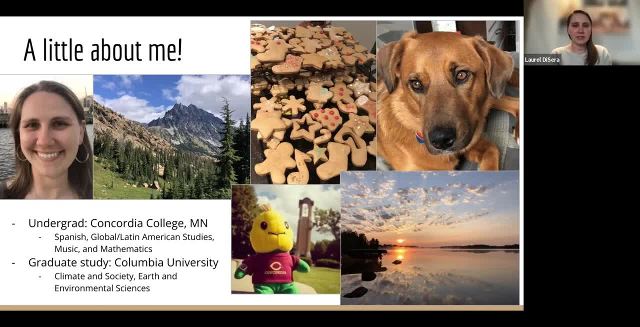 I'm currently doing my PhD in earth and environmental sciences. Now, outside of school, I have a lot of interests. I like to go hiking, I spend time in Minnesota in the land of 10,000 lakes, And I like to bake, and that's my dog. 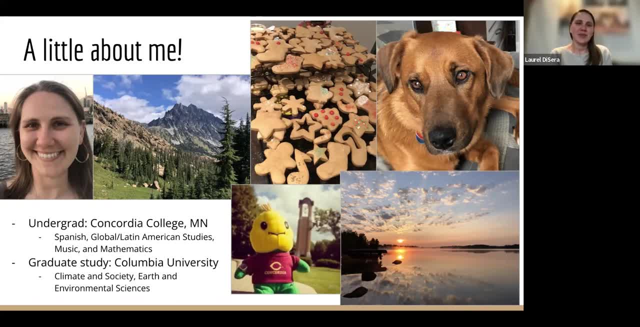 Perry. So hopefully she doesn't make too much noise, But if you hear a bark you know where that's coming from, coming from her. So that's a little bit about me. I'm happy to answer any questions that you have about college or my journey to college. 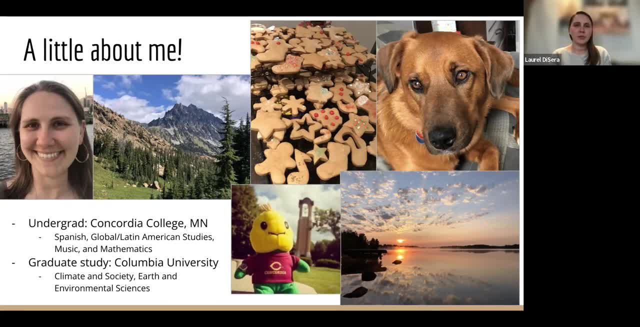 So that's a little bit about me. I'm happy to answer any questions that you have about college or my journey to climate science, because it's a bit abnormal compared to some of the more traditional routes, But maybe we can talk about that about that at the end. I will be monitoring the chat during this presentation. 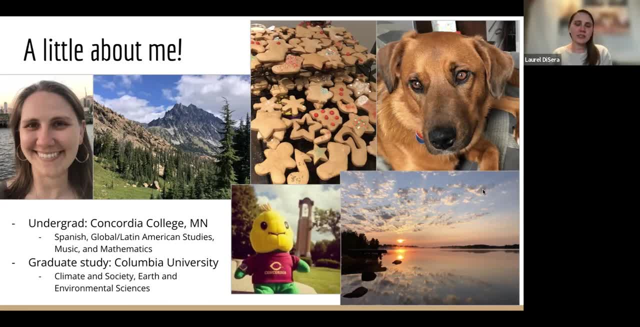 So when I ask questions, feel free to respond in the chat And if you have questions for me, post them in the Q&A so that they don't get lost in the chat with all of the different things happening. So let's talk about symphonies. 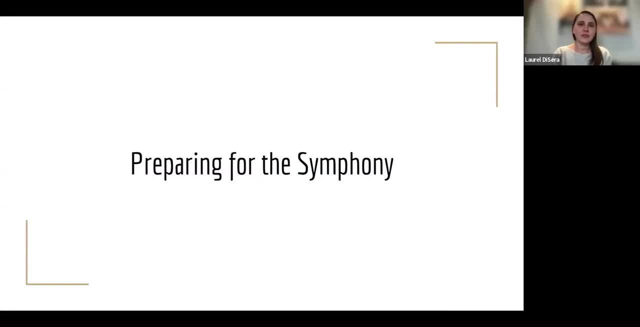 So let's talk about symphonies, or preparing for that by sort of early days as well as later, wohlweiner into the future, our symphony, And to do this we need to talk about what a normal symphony is. So just take. 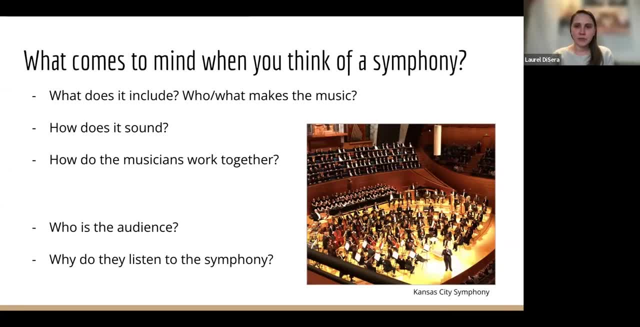 a second think about some of these questions And if you have an answer to any of them, feel free to post them in the chat. We're going to go through and talk about them. So we're a little bit more prepared to talk about what a symphony might mean in the climate sense. But you probably have 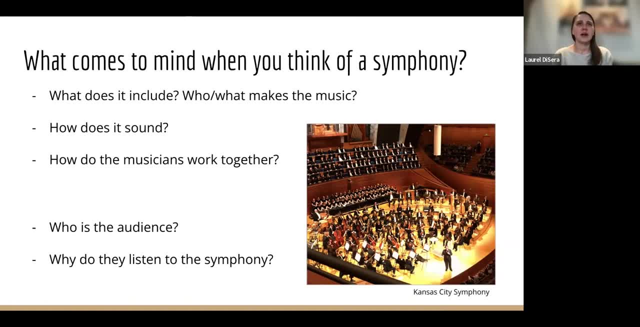 all heard of a symphony or an orchestra or a band, or even a full choir, So if you have been in any of those, what do they include? Do they include instruments? Do you play an instrument? How do an orchestra or symphony or a band sound? Do they sound harmonious? How do the musicians work? 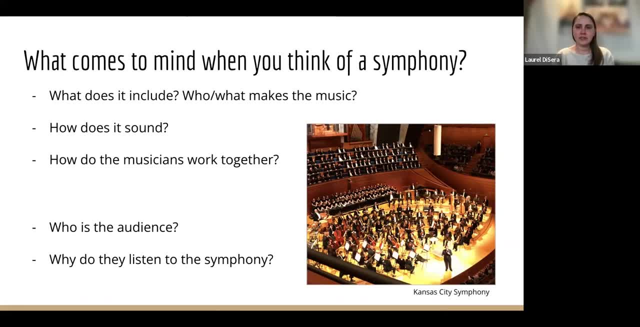 together And who is the audience? Does anyone have any thoughts or examples of music? Do any of you play instruments? No, not too many. Well, I personally used to play. I do sometimes still, but I play the flute and piccolo, And I played flute and piccolo in college as well as in undergraduate, And that 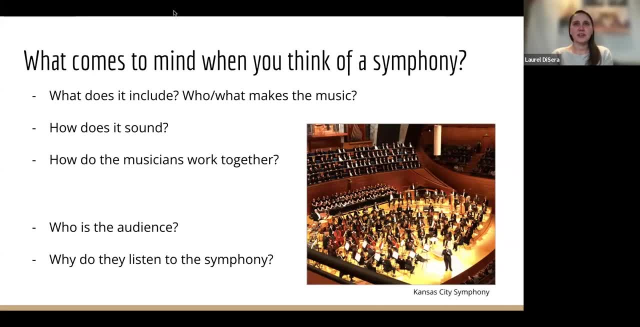 was really something that I participated in a lot of groups and it took a lot of my time and a lot of my sleep, but I really enjoyed it. So if you have any questions, feel free to post them in the chat. Any thoughts on instruments or things that make your life fun in an orchestral or symphony? 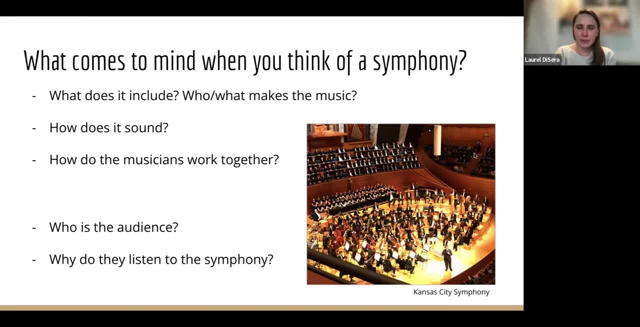 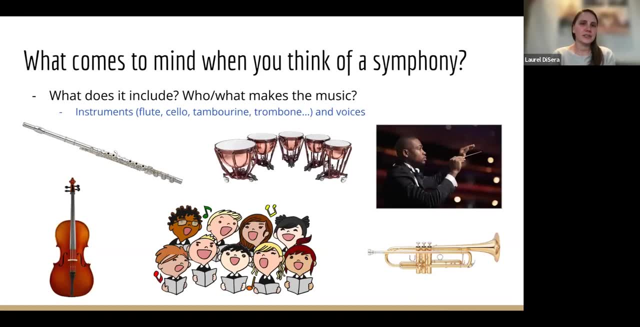 setting. please include them in the chat. But some examples that we like to think about when we think of who makes up a symphony or an orchestra include a variety of instruments, For example, a cello in an orchestra or a flute in a band or orchestra. You have timpani drums. 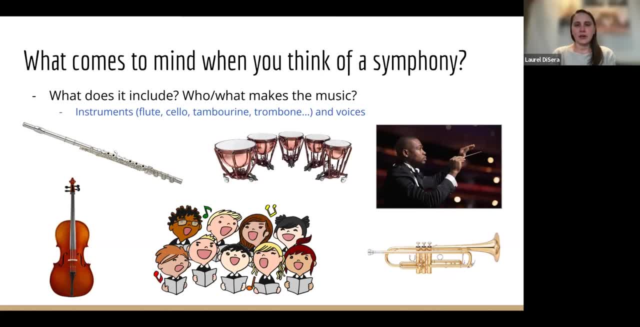 You have trumpets, cornets, trombones, saxophones, even if you're in a normal concert band, But sometimes you can have singers, depending on if you're playing Handel's Messiah, for example, or other pieces that might require singing. But the one thing that's always constant is the director. 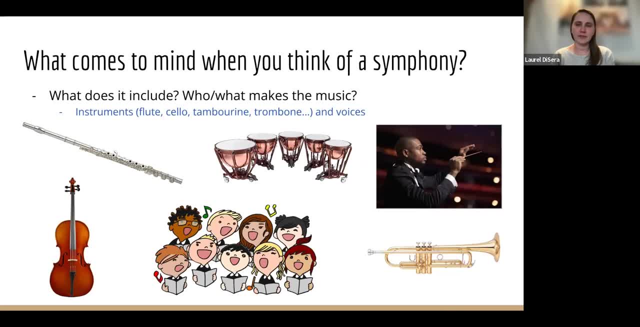 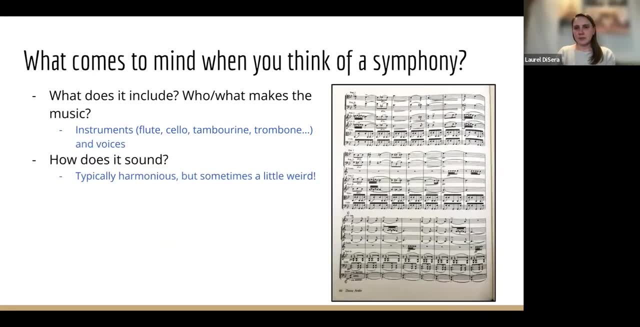 Most groups, whether they're big or small, like to have somebody that leads them, And that's really important in keeping people on the same page. So a symphony typically has different types of sounds. They can be harmonious, but sometimes they can be. 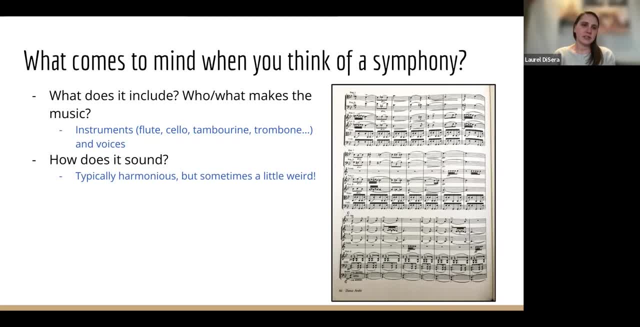 dissonant And we often need these dissonant parts to make the harmonious parts more worthwhile. right, You have to have the ups and downs to be able to appreciate some of the nice, very triumphant parts of music. But some parts can be a little weird and might make you uncomfortable or make you nervous. 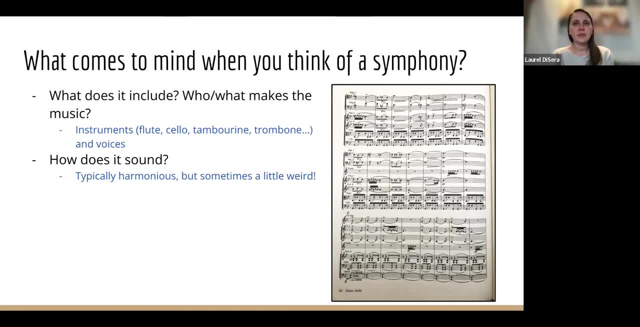 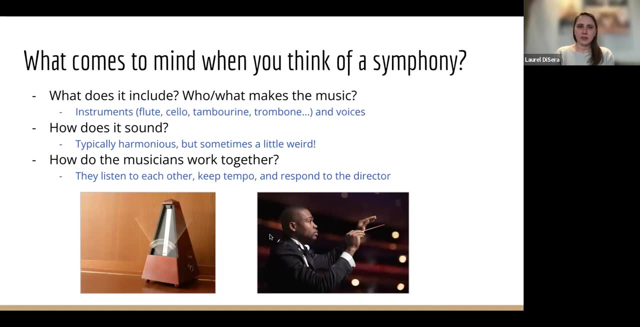 Or make you scared or sad, But that's the beauty of music And something that we also will think about when we're thinking about the climate system. And then we also think about how the different musicians work together, how they listen to each other. 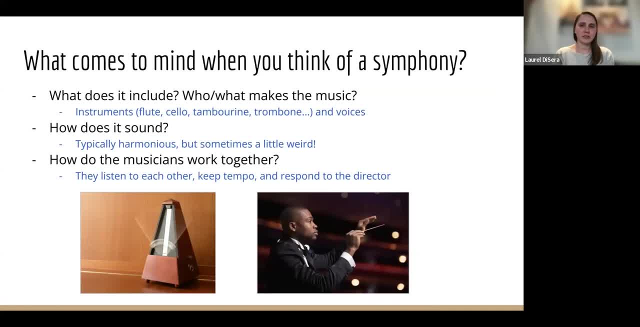 They keep tempo, maybe with a metronome, or how they respond to their director. Maybe they're watching their director's movements, looking for different crescendos or cues that might encourage them to do something different than what they see on the page, for example. 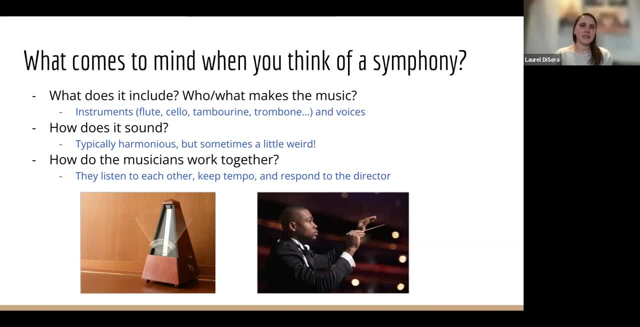 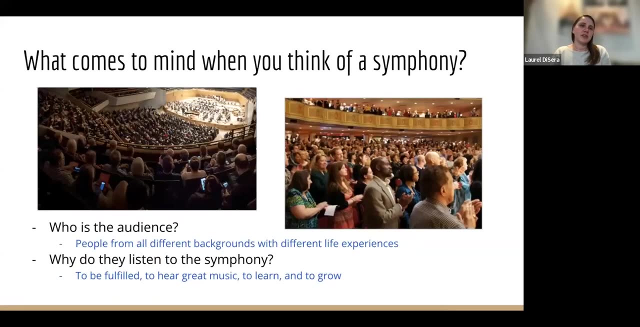 So this is a way that the musicians can play together and work as a team to create the sound of the music that is expected by the director, or how the music was written to begin with. But then we have the other flipside. We have all of these people like you who are coming to this as an audience- all 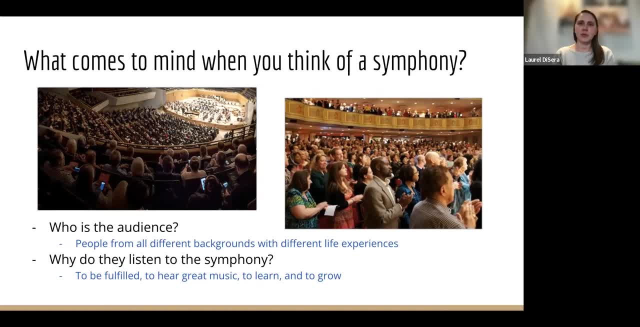 um symphonies or orchestras usually have concerts where they perform, and people come from all over the place, from different backgrounds and different life experiences, to listen to this music. um, often they'll be fulfilled, they might be moved emotionally, they may cry, they might be very joyful. 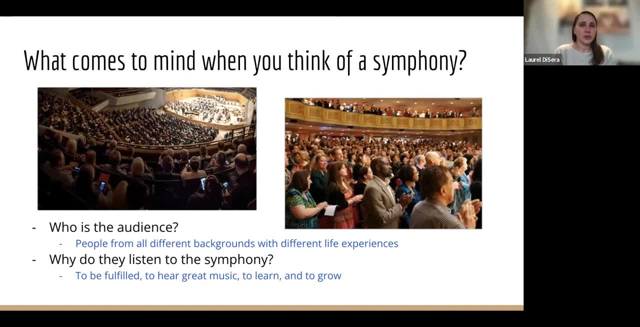 when they hear this music, depending on what's played, they'll probably learn something and potentially grow in their music endeavors, whether they're just listening or they're playing when they listen to this music. so the audience in a symphony setting, in a concert setting, is often 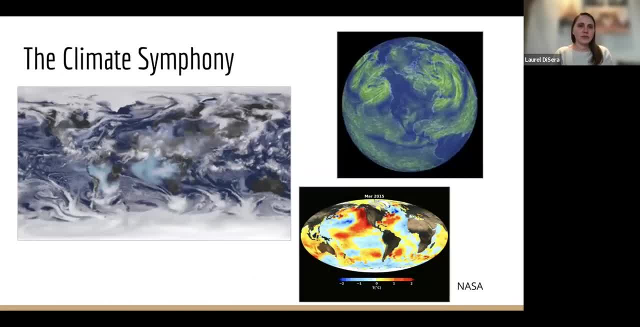 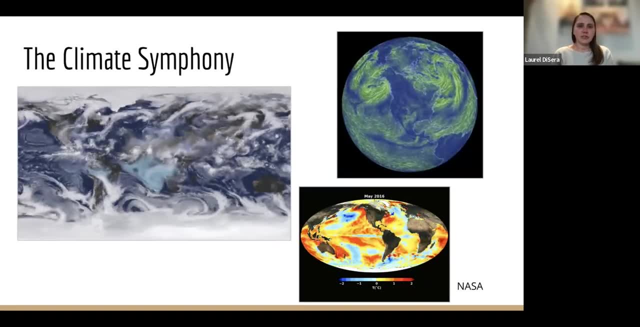 really important to think about as well. so now that we've talked a little bit about what a symphony is, in a way that you may have heard about it before- um, let's take a little bit of time to think about what our climate symphony might be. so we have a variety of things going on here that are 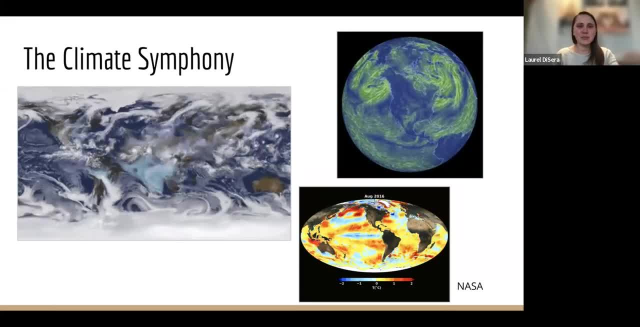 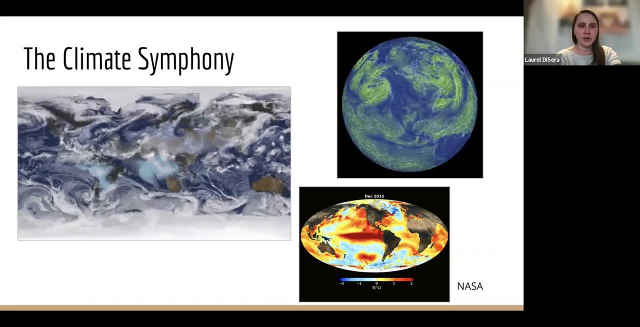 all moving and very important to us, and we're going to talk a little bit about what a symphony is very distracting. we have a simulation of clouds on the left, um, and the blue clouds are actually special, um, special clouds that are formed in different parts of the atmosphere due to 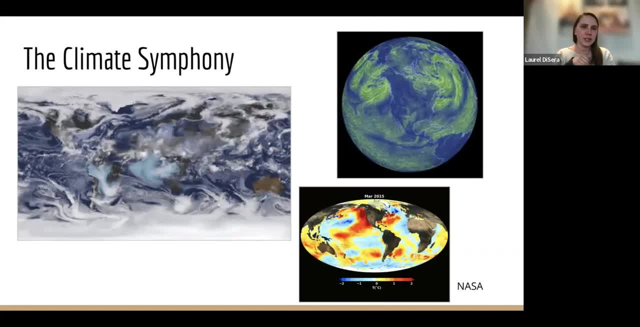 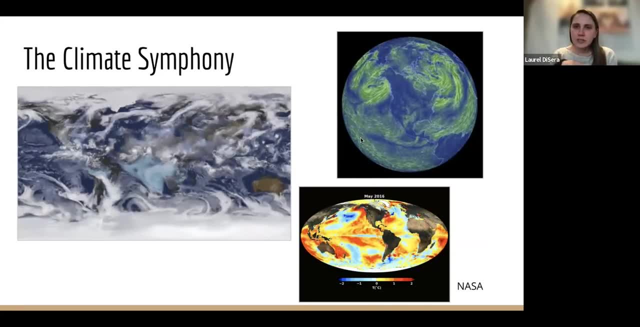 different chemicals. but you can just kind of see how the clouds move generally around the world. um, in the top right corner here we have winds. if you look really closely, those little green areas are actually moving and showing different wind patterns around the earth. um, and if you look really closely you can see that the clouds are moving around the earth. 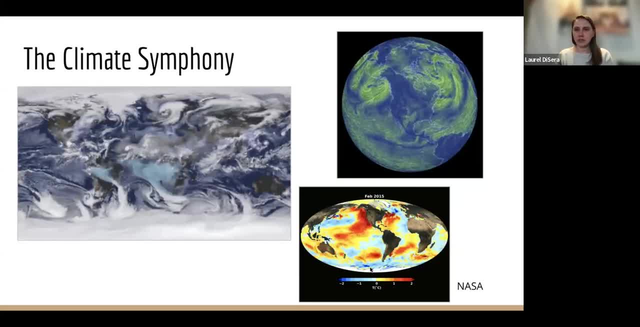 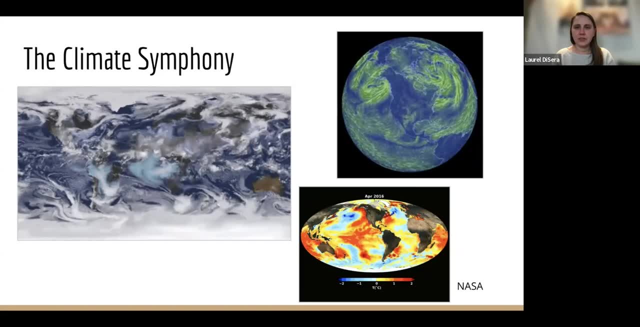 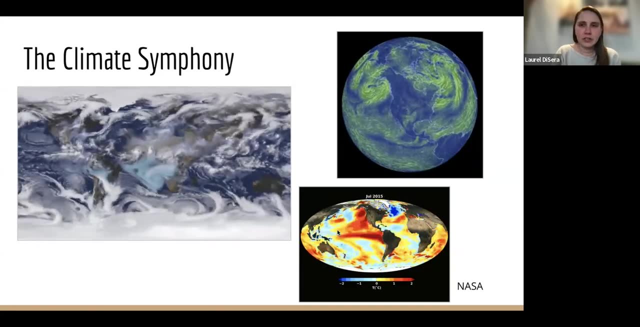 and if you look below on the bottom, you see changing sea surface temperatures. and all of these components are influenced by the earth itself and by different members of the climate symphony. so we're going to talk about a few of the different members of the climate symphony. 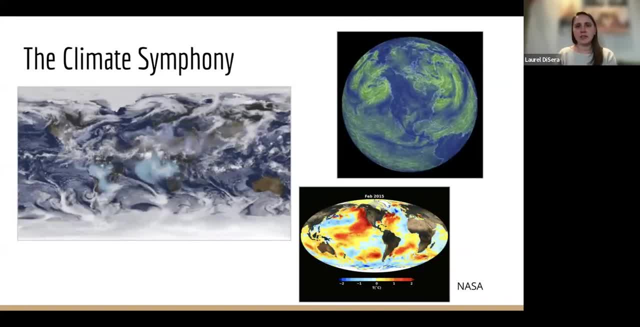 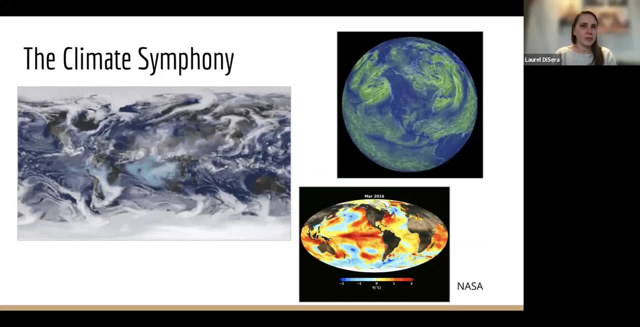 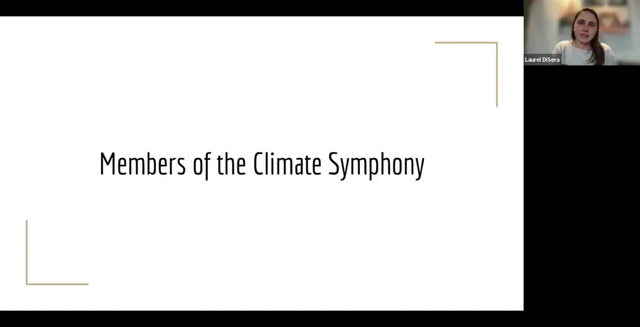 and then we're going to move on to discuss a little bit about how climate change is going to impact our climate symphony. so first um, discussing climate variability and then climate change. so some of the members, our members of our climate symphony, don't really play instruments, so to speak. 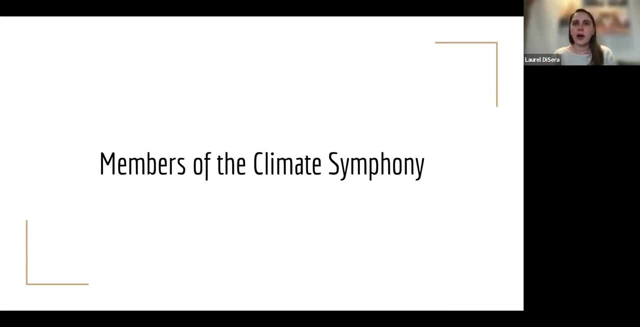 we kind of refer to them on terms of time scale or how fast or quickly they move over a long period of time, so kind of. instead of thinking about trying to equate them to um one exact instrument, we're going to talk about how climate change is going to affect the way that they move around the earth. 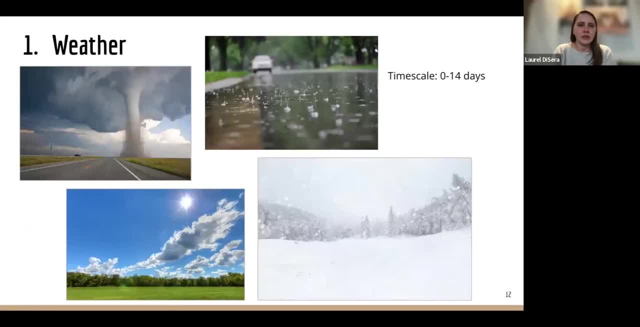 and how it affects the way that climate change is going to affect our climate and the way that we think of maybe how they can work together. so you all have probably kept track of this. you have the app on your phone that gives you the weather from day to day. 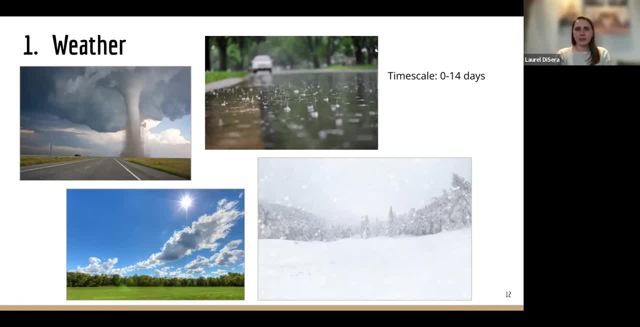 but here are just some examples of what we, as climate scientists, consider one of our symphony members, which is the most rapidly changing type of weather, their type of climate symphony member, which is weather weather. There are tornadoes, there are thunderstorms that bring rain, there are clear 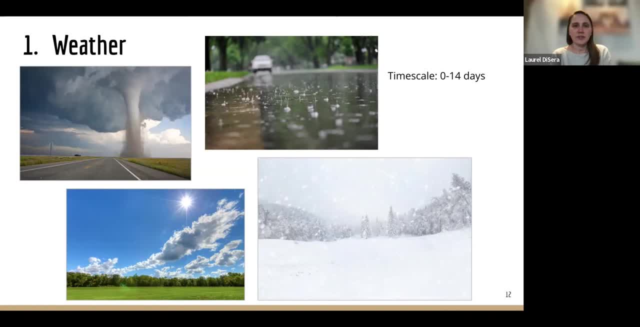 sunny days and there are also blizzards. Granted, if we all live in the New York area, we know that there haven't been too many blizzards down towards Manhattan. Does anyone have any other ideas of other types of weather that we may experience other than snow and rain and sun? 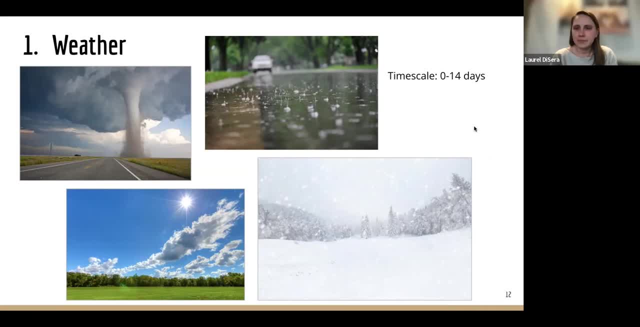 You can feel free to post them in the chat. There's like literally no wrong answers Right now in New York it is sunny, I think it's mostly clear sky. I haven't been outside for most of the day, but it looks like it is a nice day out. Yesterday was really windy. I'm not sure if anyone 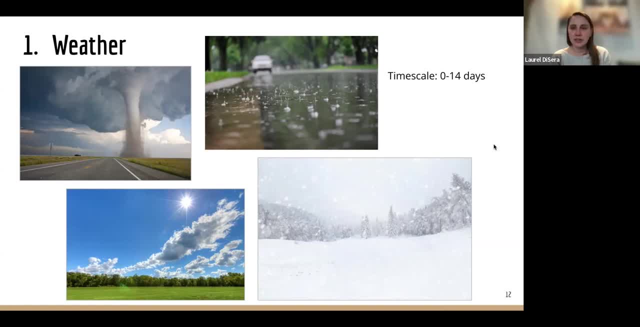 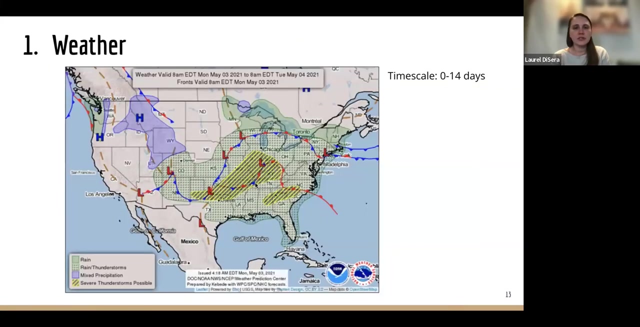 was around or walking outside and experienced that, but it was quite windy out Blowing away things that I saw. So weather is moving pretty quickly. We see that weather changes. weather patterns change from day to day. right, You may have seen something like this on the news if you ever watch the news. 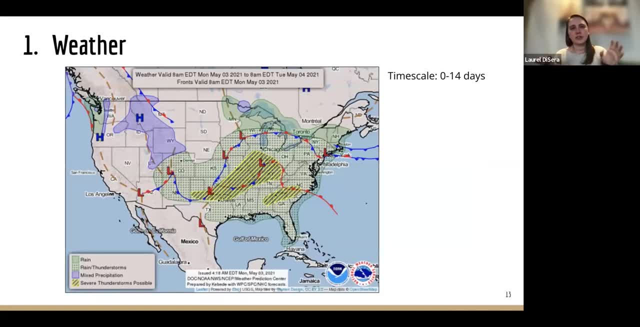 Maybe a map that looked kind of like this that looks at low and high pressure systems, And the map, similar like this, helps to inform weather people- weather men and weather women on the television- and help them explain to others what they're seeing. We've seen a lot of weather events that kind of show up and help us when we might be experiencing. 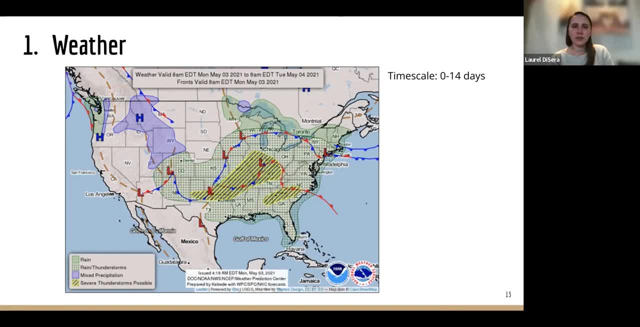 rainfall, for example, or a thunderstorm as it progresses over the United States, And we've gotten better with forecasting from what we used to be. But you know, probably on your app, on your phone, you might not want to trust something that's more than five days out for. 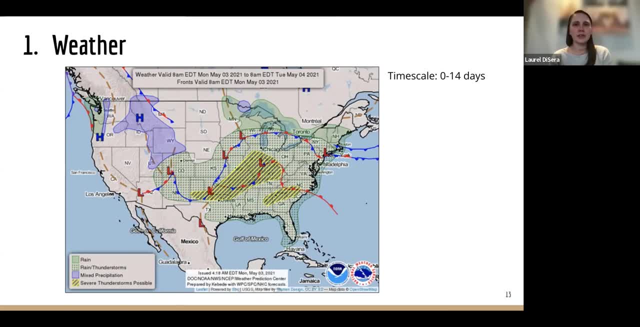 example, Mm-hmm, And meteorologists are still working on getting our forecasting to be more up to speed and more useful for people to be able to plan picnics in the park for next weekend, for example, or going to a particular sporting event that's outside. So all of this is really important. 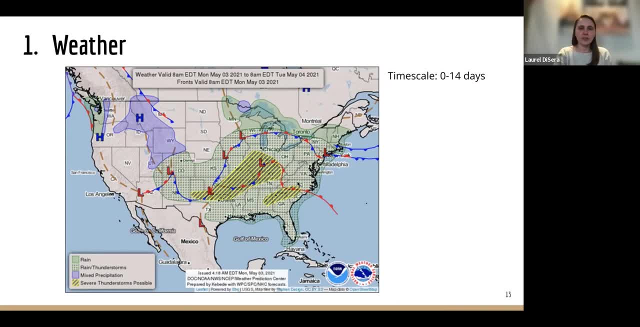 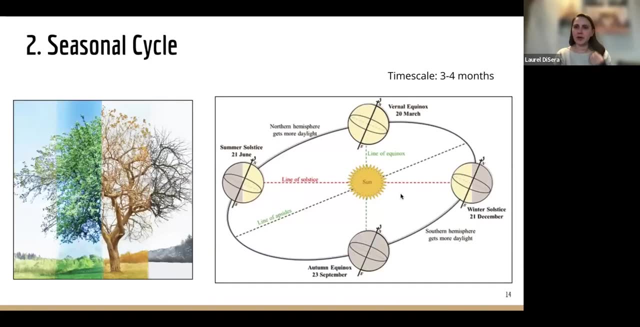 for us to understand for the day-to-day. So this is our first climate symphony member. Our second member- you're probably also all familiar with This- is our seasonal cycle. From spring to summer, to fall to winter, we see changes in our climate And this is primarily due. 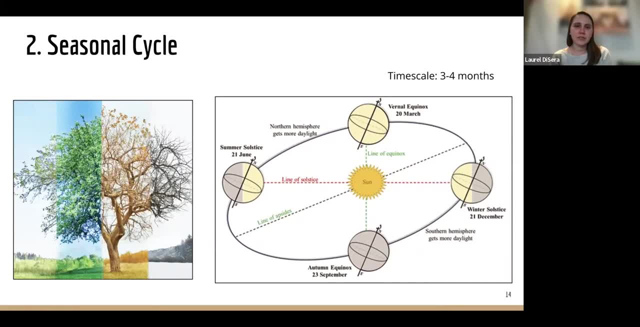 to how our earth is positioned and moves around the sun, Which part of the earth is experiencing more direct sunlight or less direct sunlight during the year, And that well, that will influence our summers and winters, And that is opposite. So we need to keep in mind that our sun is primarily guided by the sun in the southern. 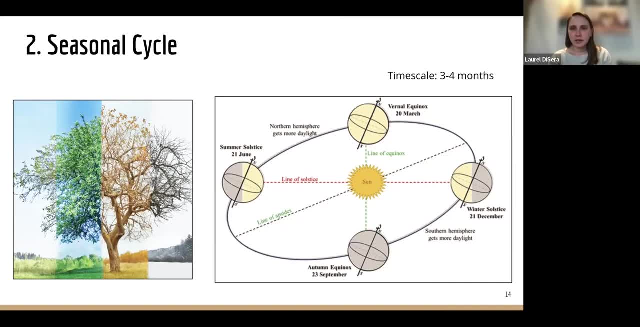 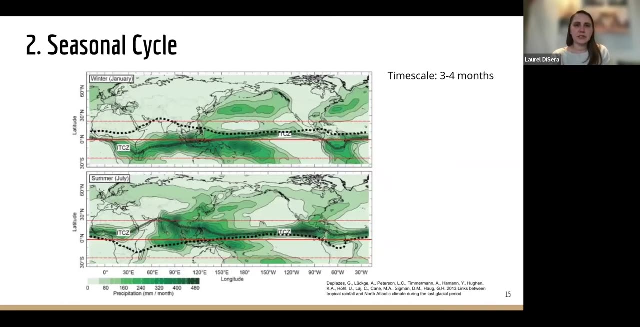 hemisphere. We can talk more about that later if you have questions- but it is primarily driven by the sun, And the sun is also really important because it heats different parts of the earth as it moves throughout the year, And this impacts how our rainfall changes. So from 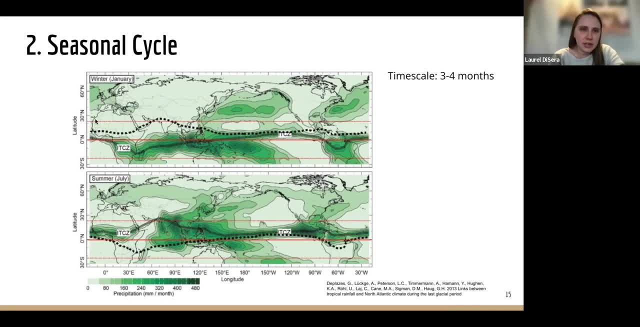 season to season, we're going to see rainfall changing across the globe. we can see of rainfall on the earth On the left side, here is Africa that you can see, and here is Europe and Asia and the Pacific Oceans in the middle, and then we have North America. 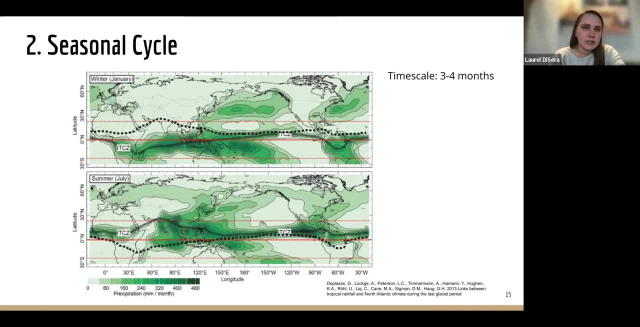 In this top panel we are looking in January and the second panel on the bottom, we're looking in July and the dark green colors are showing where we have the most rainfall We can see in the winter. all of the rainfall seems to be, most of it seems to be south of the equator and some of 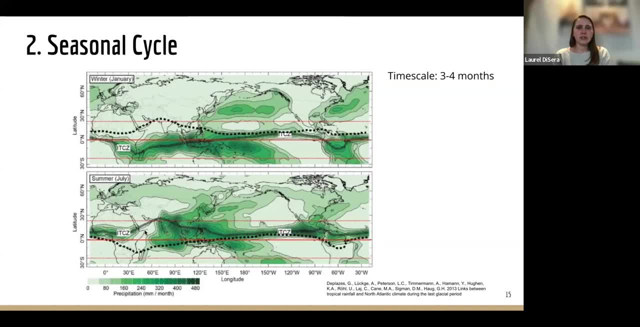 it appears to be north of the equator, and this has to do with where the sun is and how warm the water is that the sun is shining on. So our seasonal cycle and how closely we are facing the sun, for example, can impact where our rainfall changes, where it can be stronger or it can be weaker. 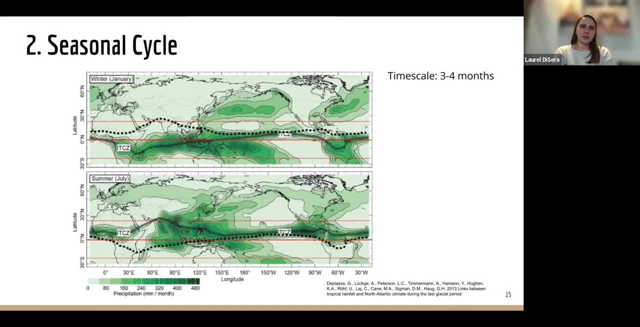 So the sun and our cycle around the sun is another really key, important player in our climate symphony and it changes. obviously we're going to have a full completion of it every one year, but you're going to see changes every three to four months or so when you're potentially closer to 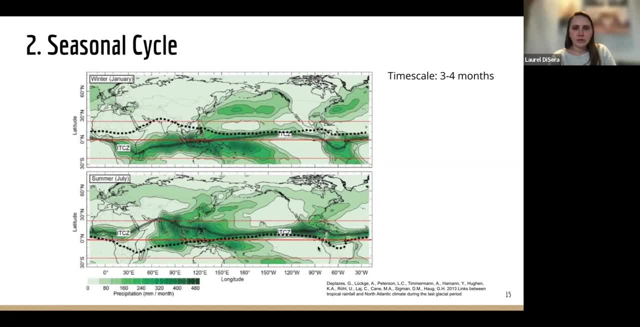 the equator. this like bold red line here. So these are weather and our seasonal cycle are probably most common and what you probably learned about in school prior to this presentation, But we're going to talk about a few other climate symphony members that might not be as familiar to. 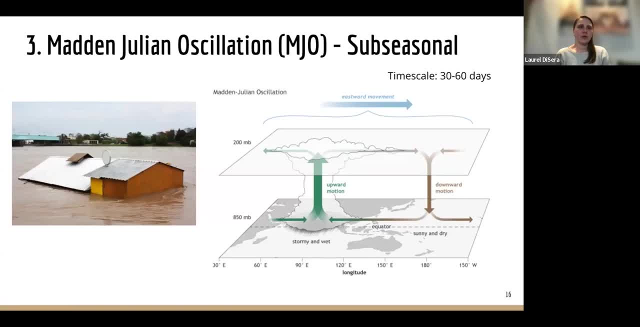 you. So the other, one of the other climate symphony members that you are just going to meet is called the Madden-Julian Oscillation, And the Madden-Julian Oscillation is essentially this like think of: if you're looking at this slide, you're looking at an look this way, like this: 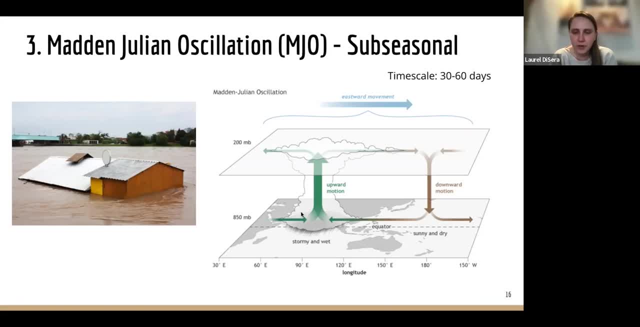 diagram here. it's like really stormy weather over a particular region that then forms clouds and it rains, and then we have dry air that sinks down because it has no more water and creates dry, sunny areas in a different part of the world, and these stormy, wet areas can cause major flooding. 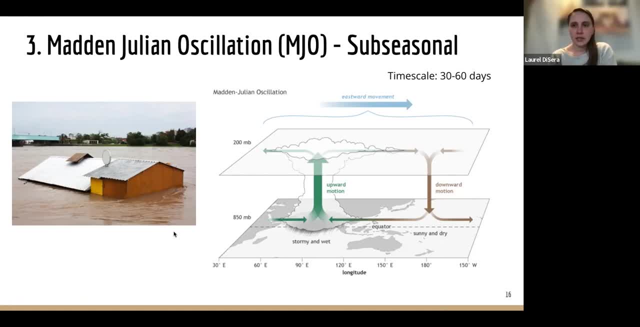 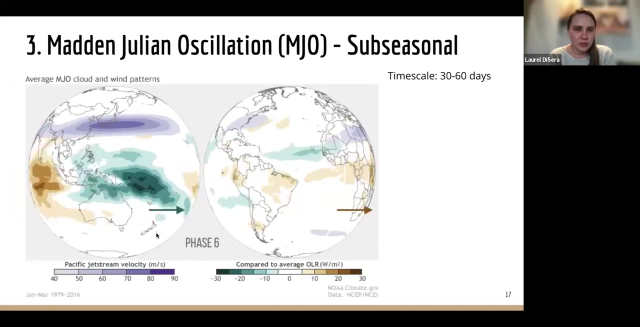 and something is something that scientists really have to keep an eye on because they need to be able to warn governments and other leaders and decision makers about potential threats to communities. but the crazy thing about the mad and julian oscillation is that it actually moves. so if you look at these cool globe images, you can see that there are these really kind of brownish. 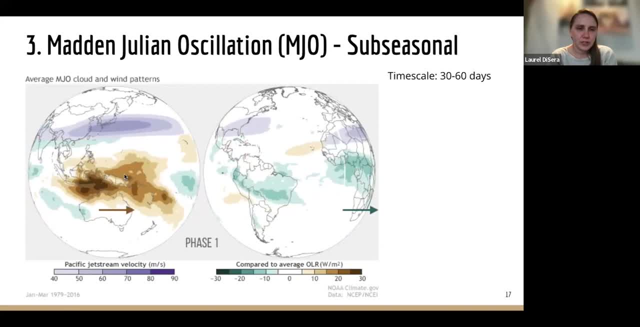 areas. just kind of ignore the problem purple parts- because we won't- we won't talk about that today, but there's the brown areas and the teal areas, and the brown areas represent dryness and the teal areas represent rain. so you can see this is Australia and then this is South America. so it's just kind of showing two different sides. 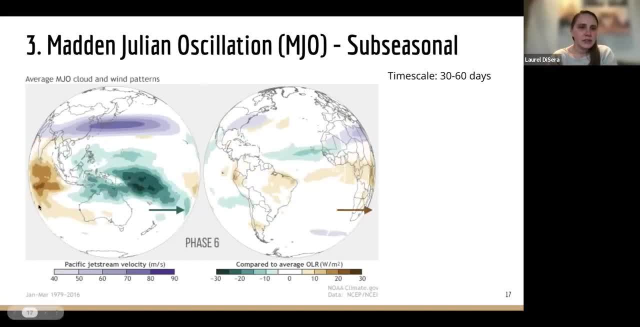 of the globe and you can see that this rainfall kind of moves towards the east and it is both followed and ahead of, or is behind, I guess, another a dry area. and this is the probably one of the more key important things about the Madden-Julian Oscillation is it moves. 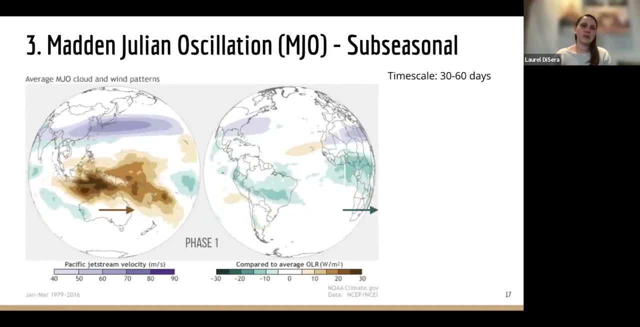 rapidly, so we have rainfall events that are moving every 30 to 60 days, and this isn't something that you can find on your weather app on your phone. this is something that we're still working on getting incorporated into our weather forecasts, so it's one of the 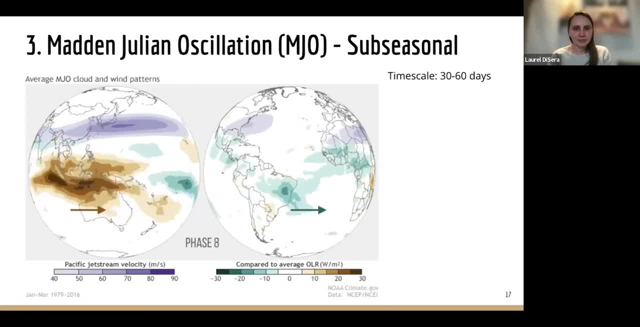 new and kind of cutting edge things that scientists are looking at today and, like I said before, if you have any questions on anything or you want me to clarify, feel free to drop any questions into the Q&A and I'll get to them when we get done talking about. 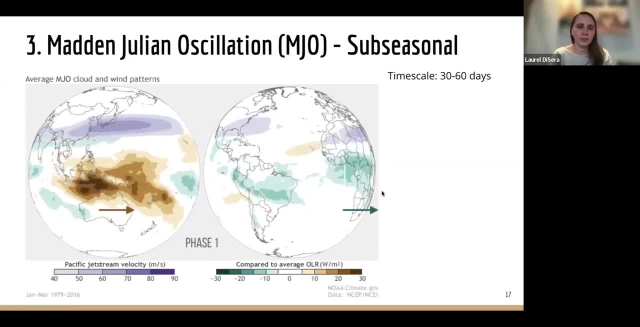 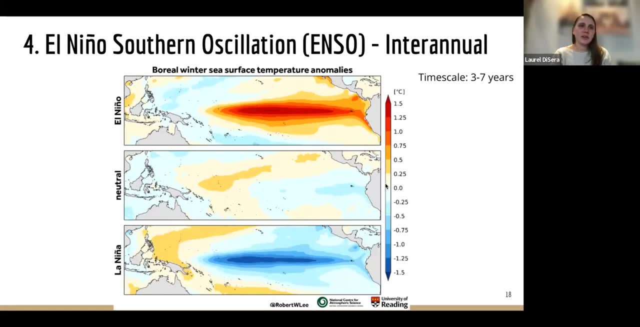 our different climate drivers and or our symphony numbers. I guess we could say um this one, however, you may have all heard of um. this different type of climate symphony number is called El Nino Southern Oscillation and it occurs on a time scale of every three to seven. 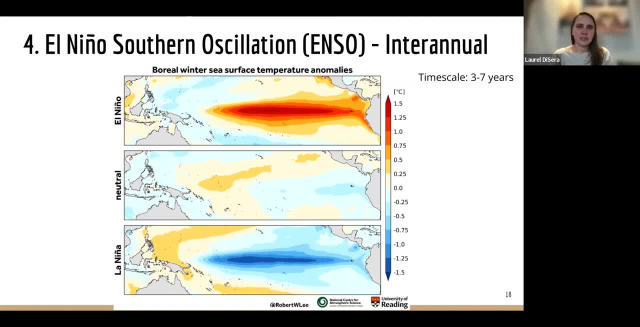 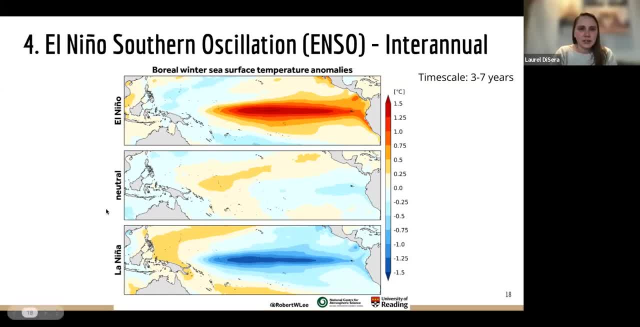 is the Pacific Ocean. so we can see here on the left side you can see like the northern little tip of Australia and Southeast Asia, and on on the right side we can see part of Mexico into Central America and South America, well, the western part of South America. 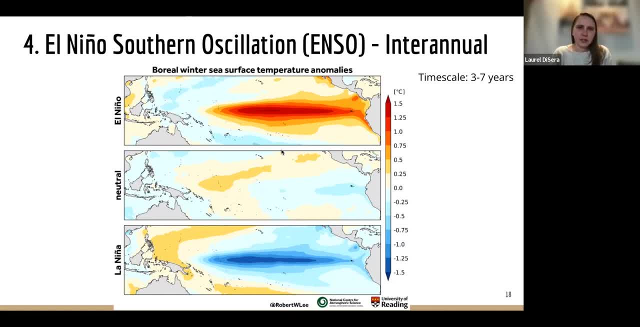 and we see that there it appears to be like three different types of El Nino Southern Oscillation. we see something with really red color here which, when we look at the scale bar on the right, we can see that this is temperature anomaly, which means if we take the normal temperature and we remove it from the sea surface, this would be the 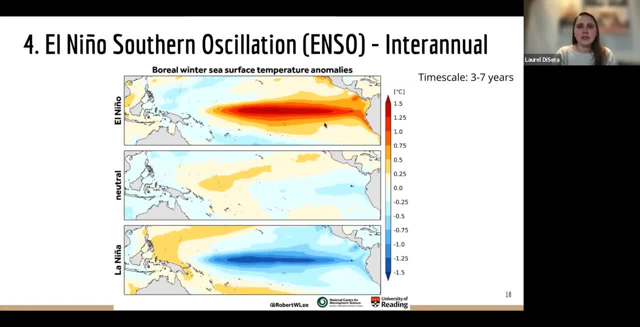 anomaly or what's left over. so we see that there's some really warm temperature here in the ocean. in the El Nino state there's a neutral state which has some warm and some cool, but nothing very strong, and then there's a La Nina state that has very cool temperatures, and these are all driven by a variety of mechanisms that we're. 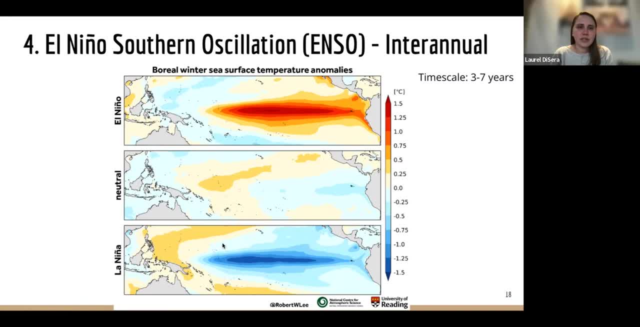 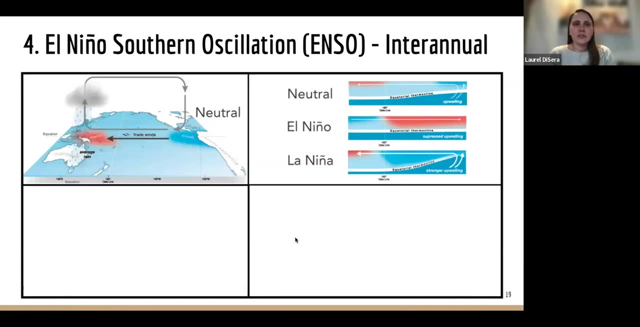 going to talk about step by step to kind of help you see how these are formed and what they can do. so to start off with El Nino, Southern Oscillation has, like I mentioned, three different phases and we're going to start with the neutral state. and then we're going to start with the neutral state. 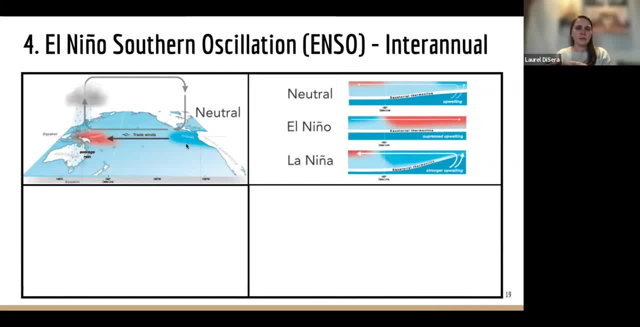 so in the neutral case, remember we talked about how the winds move and there is often rainfall- that happens in a particular region- and then drying. well, this is very similar to the Madden Oscillation, Madden-Julian Oscillation, but on a different time scale and a much larger. 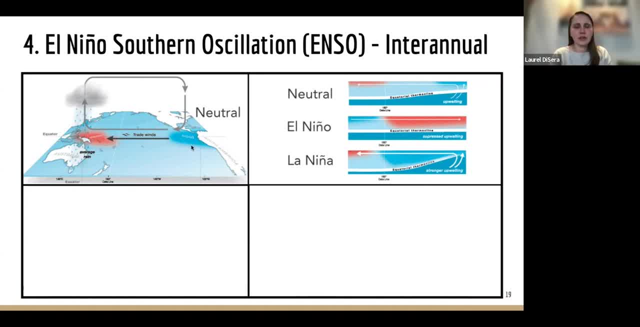 scale in general. so in the neutral time, when there's no El Nino or no La Nina event, we have trade winds that are pushing warm air and warm water over towards Australia, which then form clouds. we have um convection that forms rising air, and then we have dry air that moves over towards 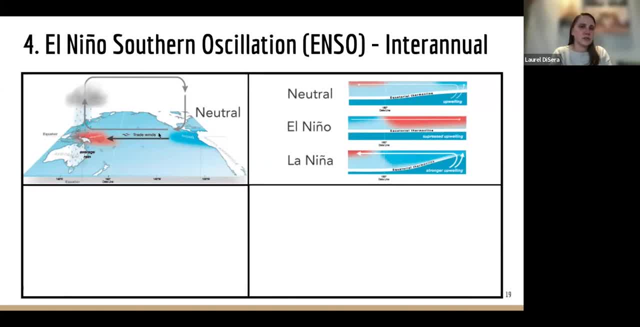 North America descends over this and descends over this cool region. so it's kind of a big cycle, um, and this is what we call, like the normal or the neutral state, And we can see if we look under the water. we can see here in this small panel what is. 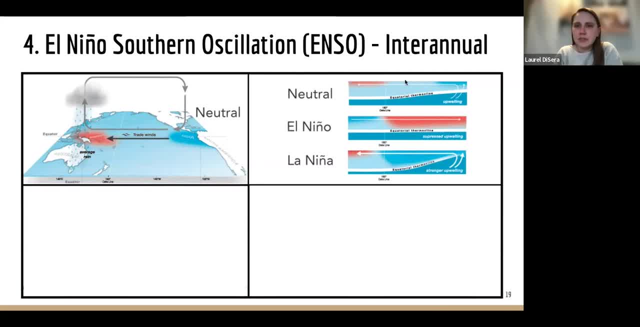 exactly going on. so we think this top part of this panel is the surface and the bottom of this panel is down several hundred feet into the water. we have this region of warm water which we see here and we see over here in the um east or western Pacific. we see this cool area here. 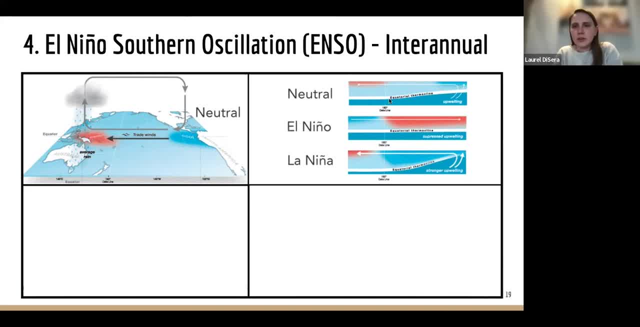 which we see here in the eastern Pacific. Then we have this thing called the equatorial thermocline, which is essentially just like this layer in the water where you pass under it- um, you pass under it or above it, and the the temperature changes really quickly. 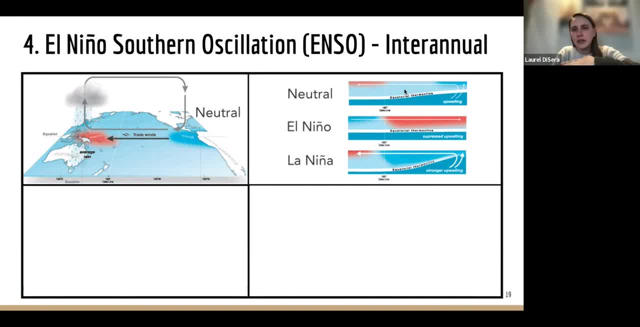 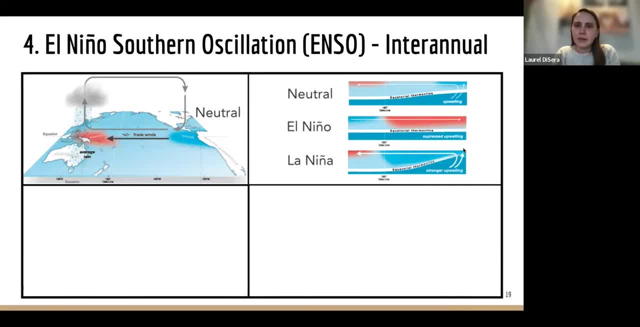 the El Nino southern oscillation, and so there are also there are two other forms of El Nino Southern Oscillation. besides the neutral, there is um La Nina, which I mentioned before, where we have a really cool section of water here over a big part of the Pacific ocean and we have really warm water over by Australia and Southeast Asia. and a lot of rainfall that has been created from the other water, enormously stronger than we have been in theunun�i Real and in tropical and landscape unnecessarily bushtog stones in Asia. so here we can see that these in these lower locations where there's extremely bright Pen comeback. why information does not stabilize high. do you wonder why? 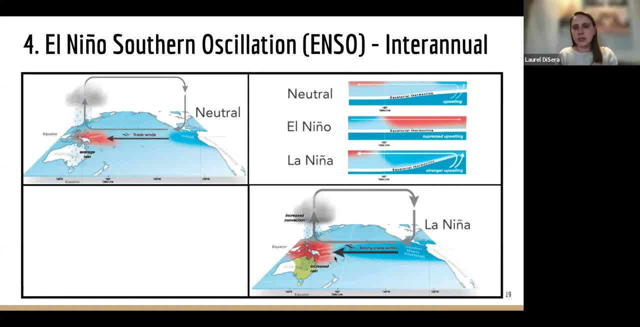 happens here. So a lot of people consider La Nina to be like a strengthening of the neutral conditions, because you have really cold water that really just gets pushed farther over than it does during neutral years. but a very similar mechanism But we see in La Nina years, for example. 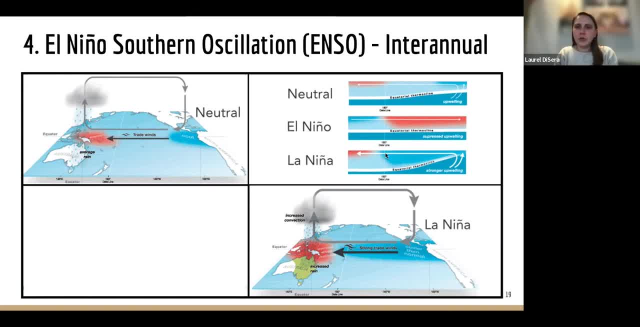 up here at the thermocline that you have a lot more cool water that's being pushed over towards Australia than you do during the neutral years. And finally we have El Nino Southern Oscillation, which has kind of a reversed pattern than what we 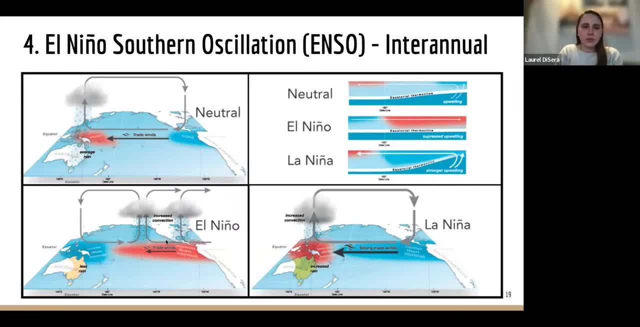 see in La Nina, starting with the warm water in the Central Pacific versus having the cool water in the Central or in the Eastern Pacific, and having more cool water over Australia and having it be quite dry And our rainfall actually gets pushed over into the Central Pacific. 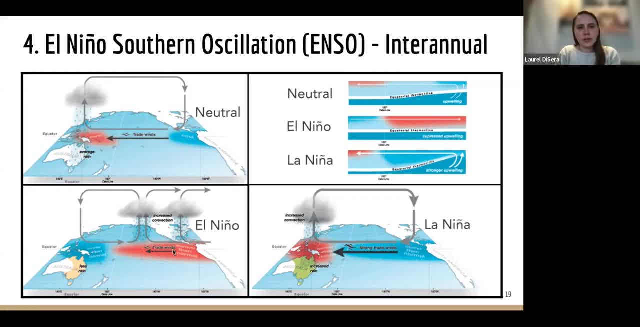 and so we have less rain over Australia and more rain over Central America, for example. We also see the trade winds also being pushed in different directions. We have weak trade winds here in the warm water and even some wind coming from the Australia area, And you might think that this seems kind of like hard to. I think 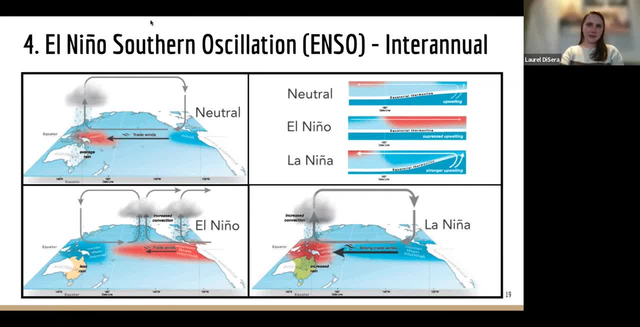 Sorry one second. Okay, I'm back. Sorry for the dog interruption, But when I started learning about El Nino Southern Oscillation, I was like so confused about how anyone would be able to figure this out. You know like this all happens over the Pacific Ocean. So how do people figure this out? 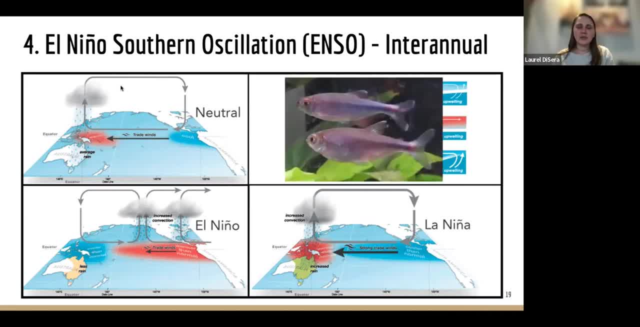 And what I was really surprised to learn about was that it really was discovered by farmers who- Well, fishermen who farmed the ocean that discovered El Nino, Southern Oscillation, because they were like trying to catch fish. But when the water temperature turns really warm or really cold, this can impact how many fish. 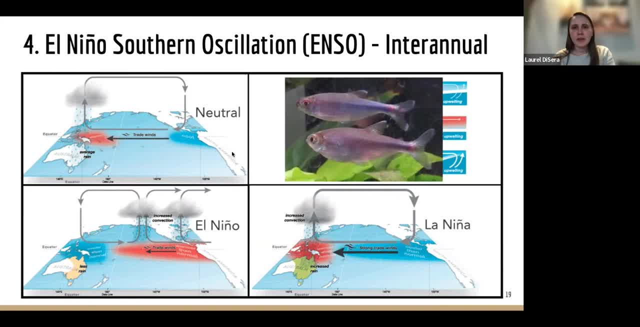 are able to thrive off the coast of Peru, And so these El Nino events will happen around December, And so the Peruvian fishers realized, around the Christian holiday, Christmas, that their fishing patterns were changing, And so they named El Nino- Southern Oscillation- El Nino because of the fact that El Nino stands for. 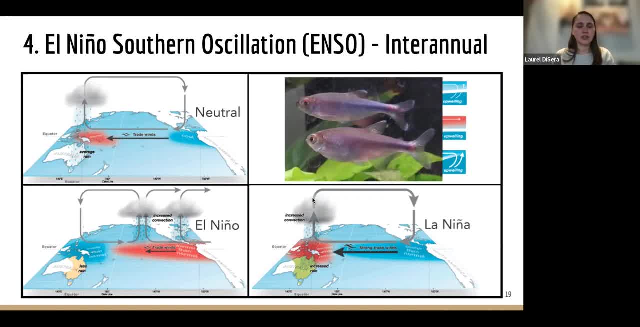 the child which represented Jesus Christ. That's how they are called, So: El Nino, Southern Oscillation. El Nino because of the fact that El Nino stands for the child which represented Jesus Christ Christ, the Christ child in Christianity. So I just think that that's really cool, that this was. 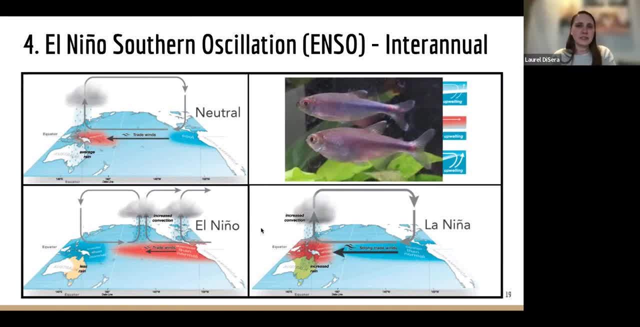 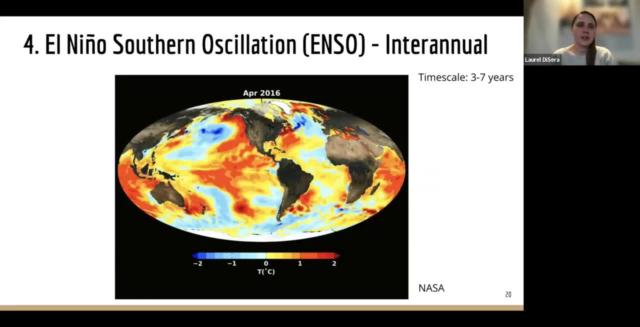 known about and studied well before any climate scientists came along to learn about it. So here is an animation that I showed earlier, but now you can kind of see and visualize what this warming sea surface temperature looks like during El Nino years and then La Nina years. 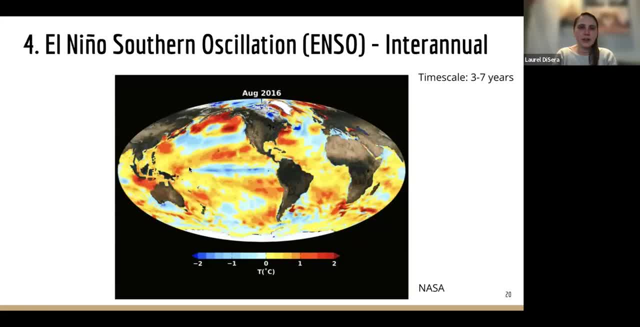 as you see, like this warm band of water here turn into a cool band of water in 2016.. 2015 was one of the largest El Nino events that we have ever experienced on earth and actually happened to be the event that happened when I was studying abroad, in Argentina, and major rainfall happened. 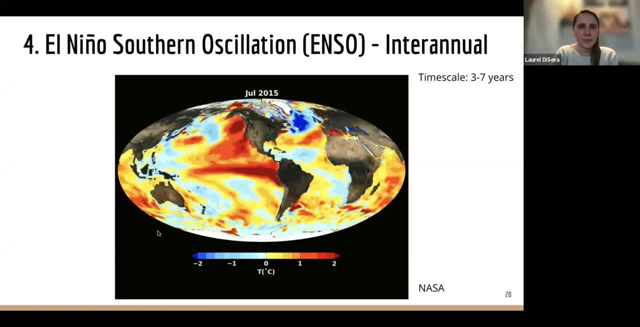 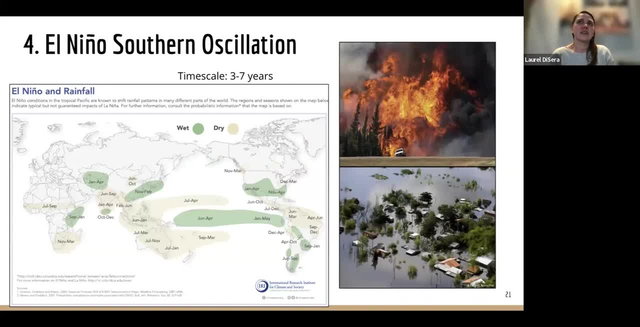 there because of this event. So it was kind of kind of cool And there's a way that El Nino Southern Oscillation is not just like impactful in the Pacific Ocean, but there's a way for us to understand how it impacts the entire. 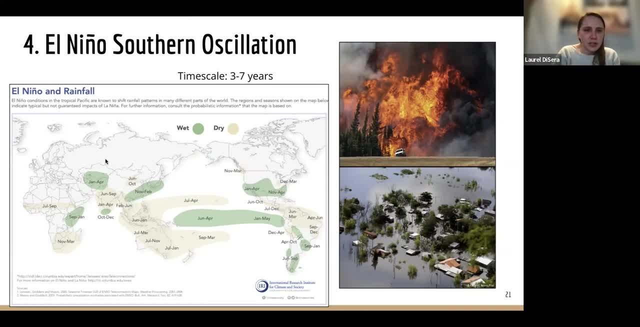 globe And we can see that in this image here. we can see during El Nino years it's drier in this brown area in some places than others and water in some places than others And in different parts of the year. so scientists study this and they understand. 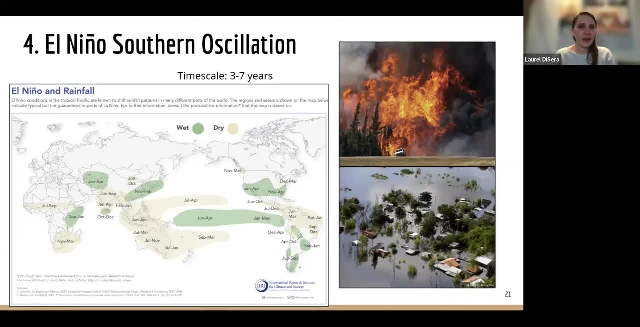 are getting better at understanding how to incorporate the water into the ocean, And so this is an image that I showed earlier, but it's kind of interesting to see how these forecasts of El Nino and La Nina into their system, so that we can better prepare farmers and even civilians everywhere for things that El Nino can bring. 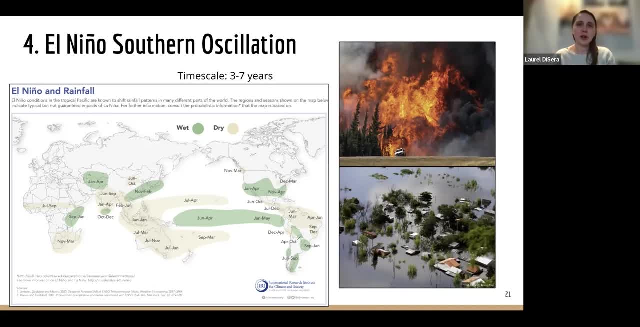 And some are good. Sometimes it can bring prosperous crop growing seasons to some regions, but sometimes it can be a little detrimental and quite dangerous, as, for example, fires which were seen in Australia during large El Nino events and also flooding in some regions as well. 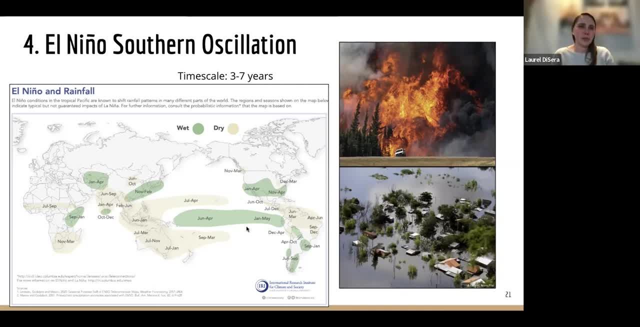 And so El Nino is another one of our climate symphony members. that happens on a little bit longer timescale, of three to seven years, But it has a lot of impact around the globe compared to some of the others that we've looked at. 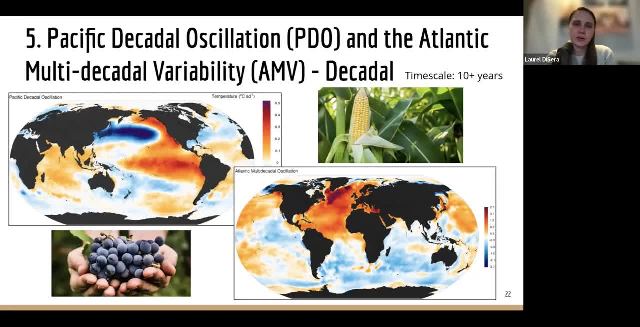 And finally two other climate symphony members. I mean there are, you know there's a lot of climate symphony members. I mean there are a lot of climate symphony members. You know that there are more than I listed for the orchestra example, But these are just a few that I thought would be. 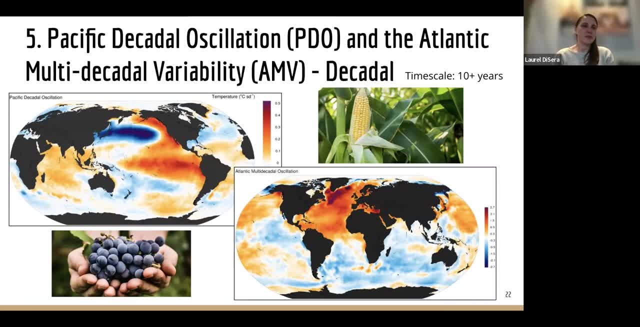 good examples. So the Pacific Decadal Oscillation is here on the right And this also has to do with the temperatures in the Pacific Ocean. but moving on a much slower timescale, We're talking about 10 or more years that these sea surface temperatures will move and modulate, so very slow. 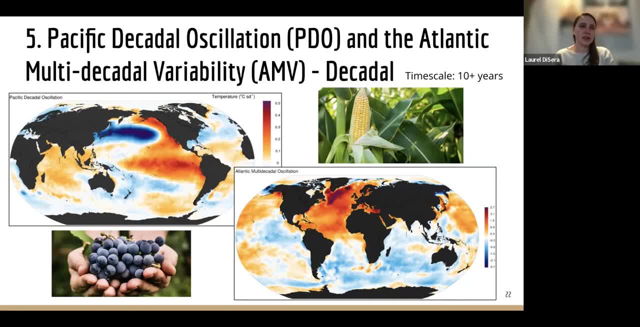 But it has a big impact on agriculture. surprisingly, These changes in the Pacific Ocean can impact grape growth in the United States and France, some of the largest grape-growing producing regions in the world, As well as the Atlantic Multi-Decadal Oscillation which has 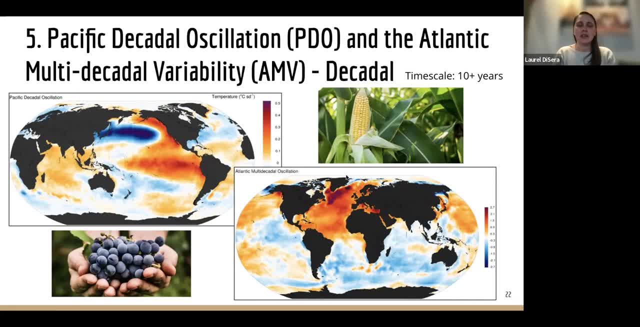 to do with the sea surface, changes of temperature in the Atlantic Ocean, And this can impact growing corn in the United States. So these changes in ocean basins that may seem far away from, for example, the Midwest can actually have a pretty big impact on the crops that we grow. and 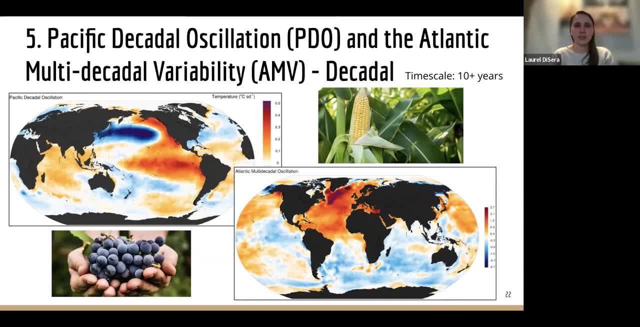 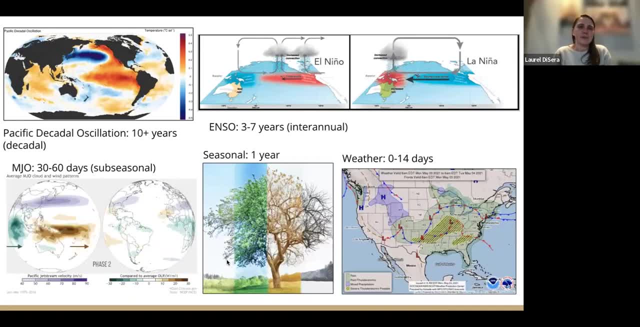 what that means for our food security all over the world, which is kind of a big deal. So when we think about all of our climate symphony members, we see that they all happen on different timescales. We have very quick timescales, like weather. We have some that are a bit longer And 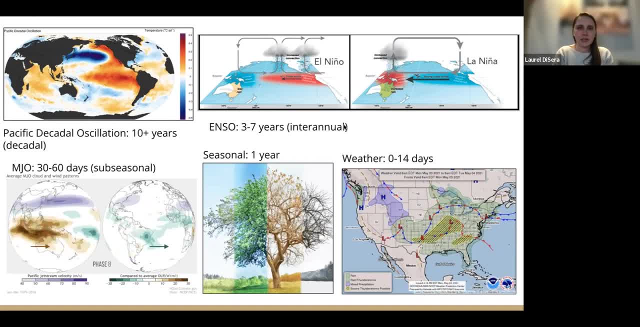 others that are really long or somewhere in between right, And understanding how they all work together is really important and is actually what I do my research on every day, trying to understand when the Madden-Julian Oscillation, for example, is over Australia and we have an El Nino. 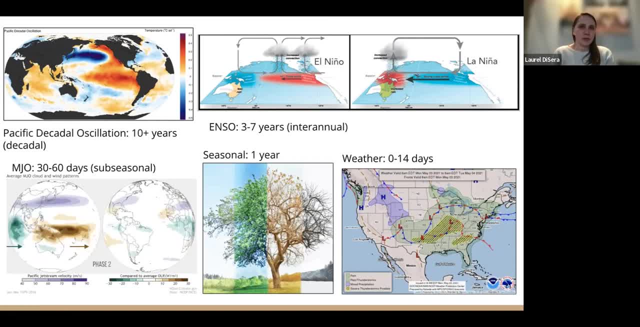 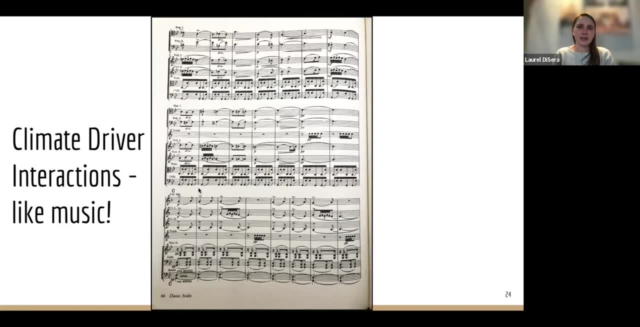 event? what does that mean for rainfall? How does that impact the people that are living there? What does that mean for their livelihoods? And this is something really important and we'll talk a little bit about it later. But to bring it back to a 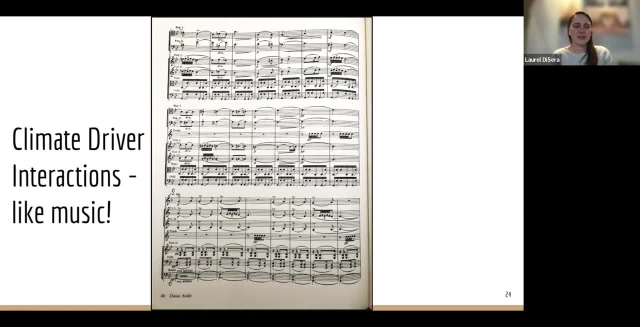 different symphony example- and this is really what I think is really a good visualization to think about- is we have a piece of music, for example, and we can assign different modes of these climate symphony members or climate drivers and see how they all kind of work together. We 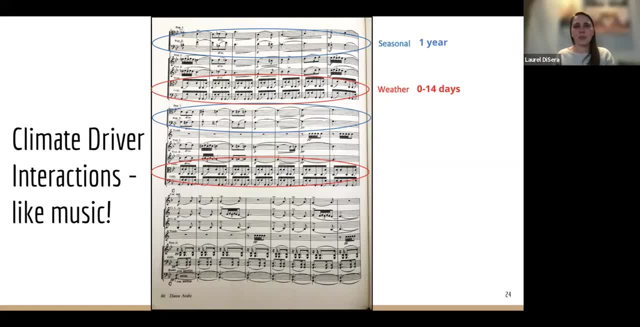 have our seasonal or something changing every three to four months, and this might be our melody that we're experiencing: our fall, our winter, our summer have weather which is kind of crazy and sporadic. it's like every other day that is changing and 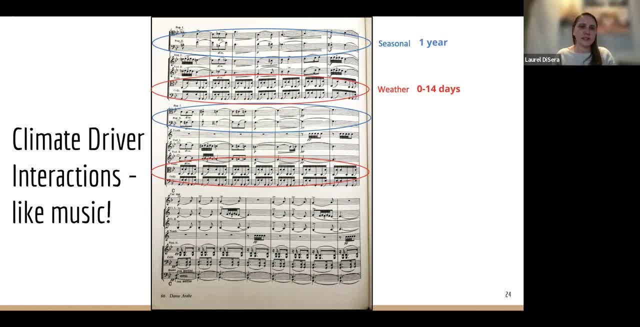 it's moving very quickly, and that might be what we find in the violin and clarinet part, for example, but we also have some slower moving drivers, and faster, depending, but more sporadic- that also contribute to this symphony of the climate, and when we play them together, we might 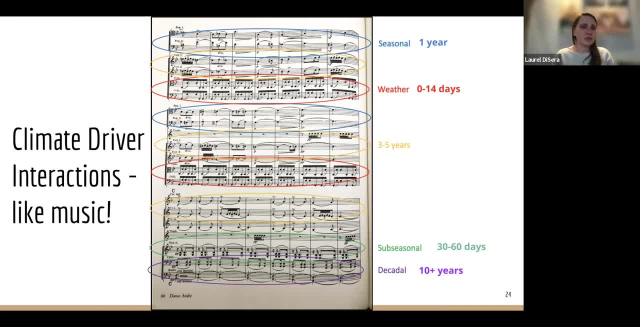 get very beautiful harmonies when we see a nice, beautiful sunny day or a season with fewer hurricanes, for example, but when we experience dissonance in the music or in the climate system, we might experience an El Nino event that's compounding with other climate. symphony members. 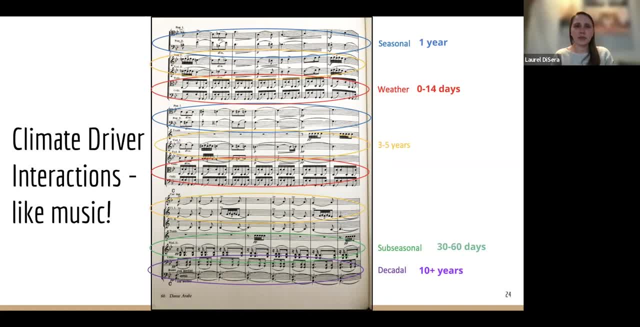 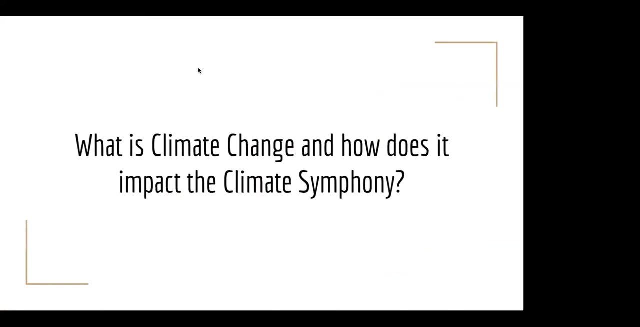 to create flooding or to create drought. that can really be impactful on society. so I'll take a little bit of a pause here to see if anyone has any questions. I don't know if there is anything in the Q&A. hey, Laurel, I haven't seen any questions come in, but I encourage you all to include them now if you. 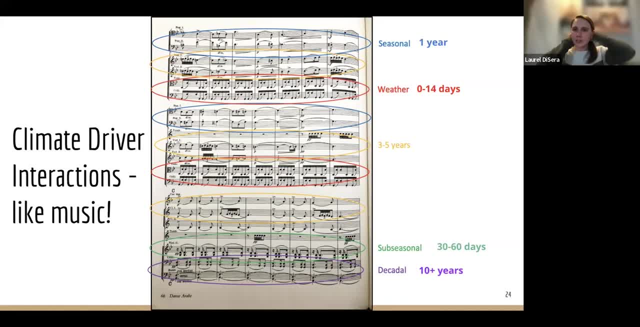 do have any questions at this time and I can answer any questions later too. it's just kind of what you're interested in learning if you have like certain questions, it just depends on what you're interested in. I can't necessarily tell you what part represents each instrument. 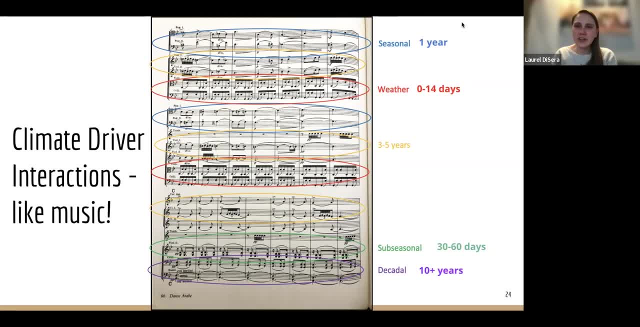 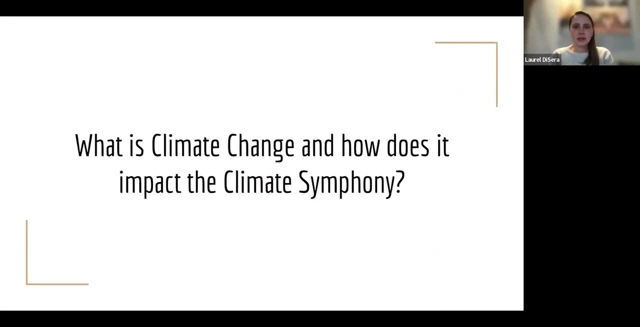 all the time, but they do change over time. so yeah, so next, I thought like it's important to also discuss how climate change impacts the climate symphony, because this is something- climate change and climate variability are often discussed, but sometimes not together, and it's really important to understand how climate variability 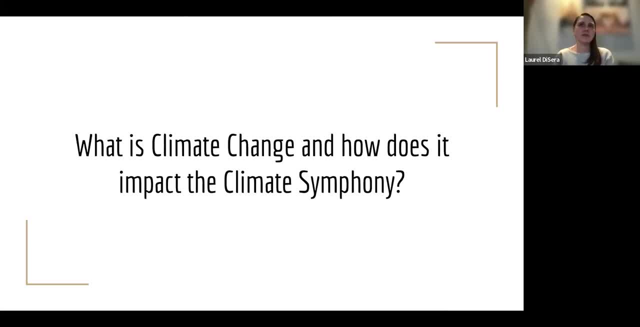 is kind of happening underneath climate change, because some events that happen in climate change or in climate variability might set off bells ringing saying, oh, climate change is causing such and such thing to happen, when really climate variability is behind it, and sometimes climate change is impacting climate variability, but it's something that we really 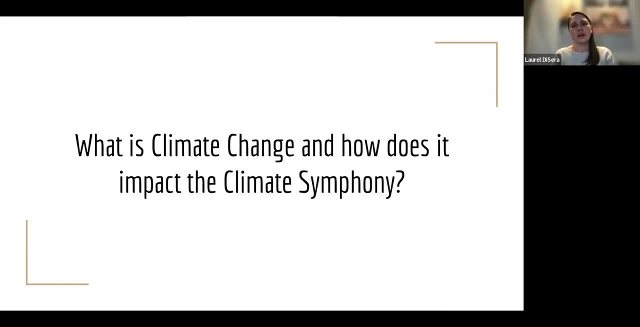 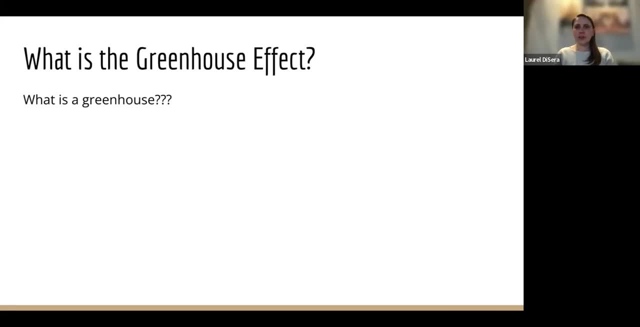 need to consider and think hard about when we are attributing specific events to climate change. so I'm not sure how familiar everyone is with the greenhouse effect and its real contribution to climate change, so I thought I would just talk a little bit about it, if you. 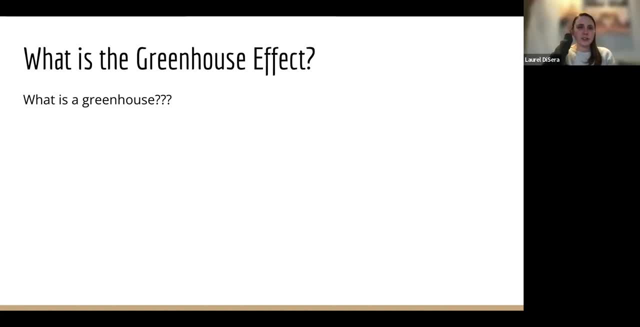 have any questions. we can talk more, but just to give a little overview. I'm not sure if any of you have been in a greenhouse. if you have, that's awesome. greenhouses are really fun. they're essentially like a building. I'm not sure I know some of the buildings in. 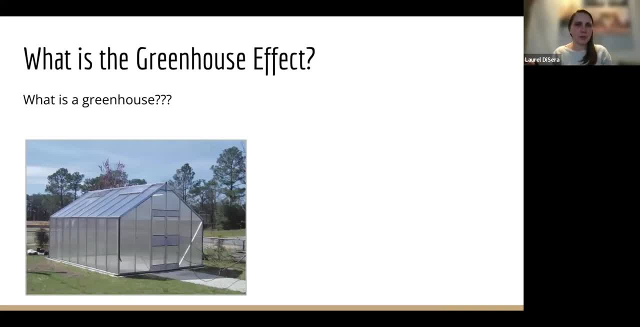 New York City have greenhouses on top of them. I've seen I think a Columbia building does and others I'm sure do, but we probably can't see because they're too tall. but in a lot of suburban and rural areas people do have greenhouses. greenhouses are a house essentially. 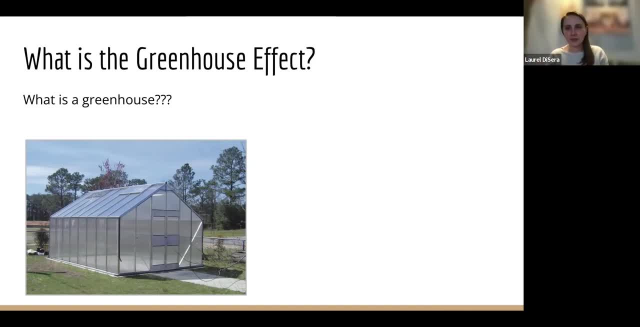 that has a structure but not hard walls. so there are no bricks that make up the house. there's no concrete or sheetrock or anything like that. there's no concrete. there's no concrete. there's no rock or plywood that make up the walls of the house. it's a transparent, can be some sort of film. 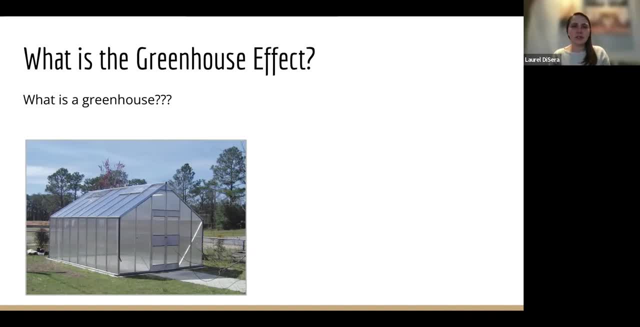 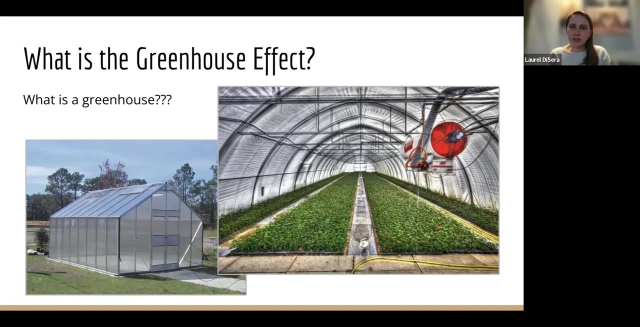 it can be plastic, but essentially the goal of this greenhouse is to trap heat, so the heat can come in through the clear walls or roofs and get trapped inside, and this allows for us to grow things even in the winter. we can grow plants on the inside and because we have this, 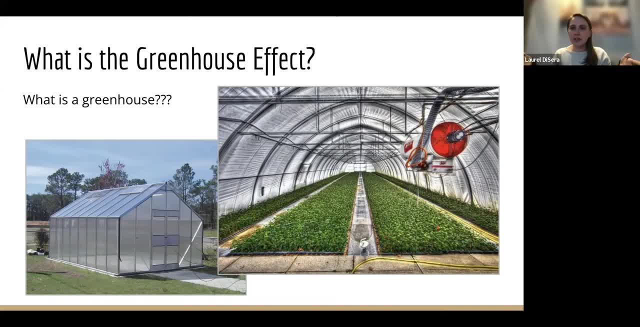 blanket of protection. we can grow plants on the inside because we have this blanket of protection here- in this case it's plastic- that can allow for us to trap the heat and grow, whether it be produce or whatever we need during the winter, and a greenhouse is essentially like the same effect. 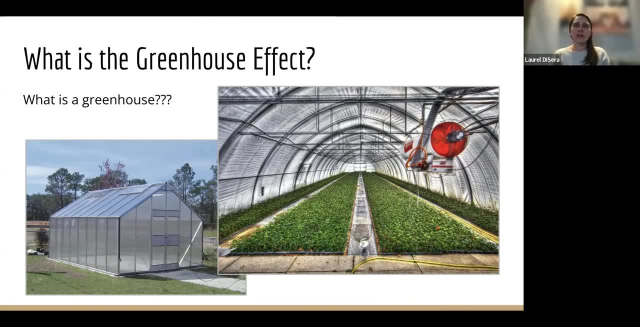 that the earth is experiencing right, so we have gases in our atmosphere that protect us from losing all of our heat to outer space. this is not the same for many of our other fellow planets, such as mars or venus. they have lost a lot of heat, they have lost a lot of energy, they have lost a lot of. 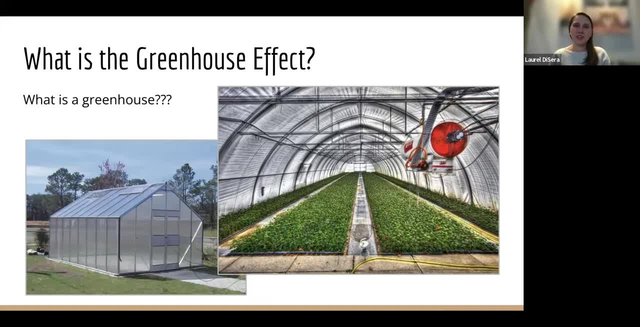 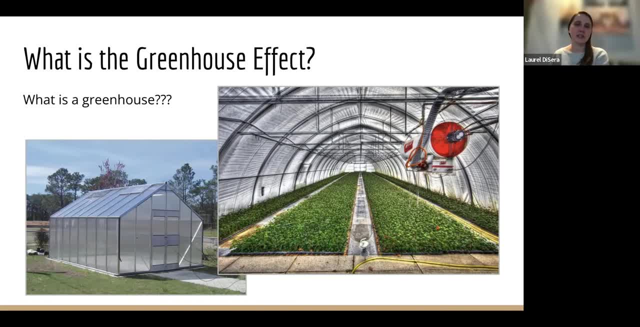 we can't go there and live there because they don't have anything to protect us and we can't give them back an atmosphere, which is also a major issue. so that's i'm not sure about. i'm not an expert on colonizing mars, but i think it might be pretty difficult. um so the greenhouse. 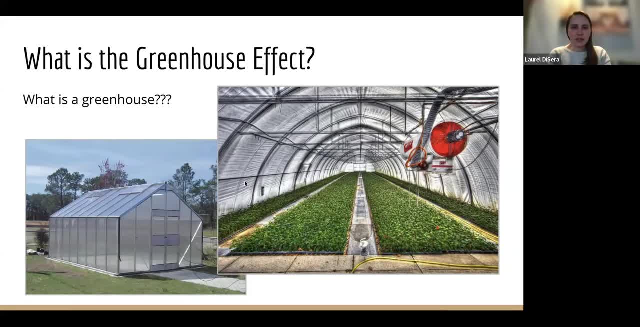 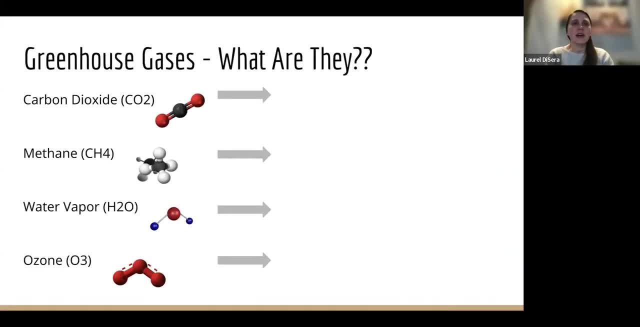 gases, like i mentioned, that kind of blanket and cover our earth. so a few of the gases and cover our earth. so a few of the gases and cover our earth. so a few of the gases that are found within the greenhouse effect, that are found within the greenhouse effect. 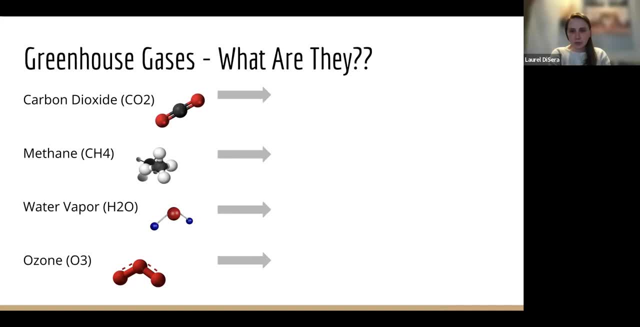 that are found within the greenhouse effect are carbon, carbon dioxide, methane, water vapor, and are carbon, carbon dioxide, methane, water vapor, and are carbon, carbon dioxide, methane, water vapor and ozone, ozone, ozone. so just to give a little bit of um. so just to give a little bit of um. 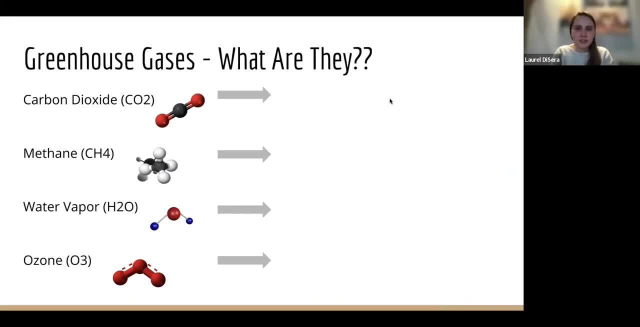 so just to give a little bit of um background to these gases, i just have a background to these gases. i just have a background to these gases. i just have a couple pictures, couple pictures. We have carbon dioxide which I'm sure you all know comes from cars, it comes from factories. 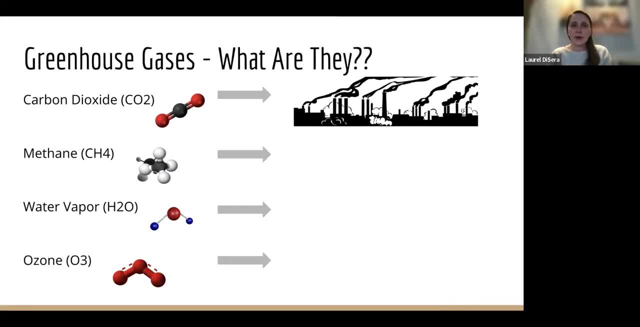 anything that works with fossil fuels, coal, anything really from within the earth, right, And this is something that we can control- that we have been pumping into the atmosphere. We have methane, which we also generally control. Methane can come from. 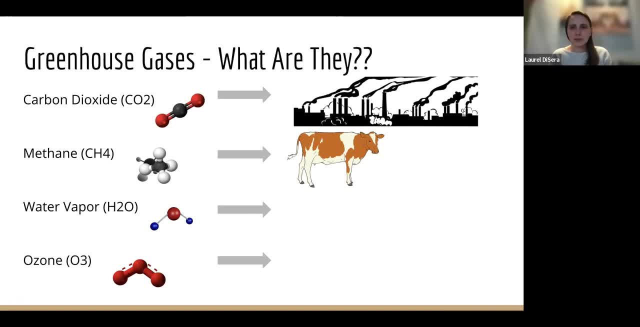 a variety of sources. probably the most well known is from cows. When cows process their food and then they release gas. specifically, from belching they released methane into the atmosphere. Fun fact, I recently learned that scientists are working on implementing in Australia a food additive for cow food. 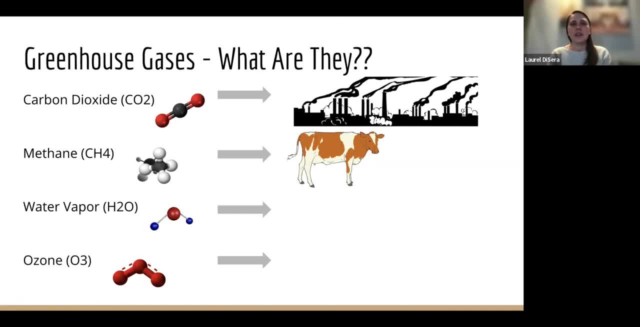 that it's like some sort of algae that they can add to a cow's food. that will reduce the methane that the cows produce in their stomachs and then release into the atmosphere. So really cool things. If you want to learn more about that, I can direct you to some information on that. So that's. 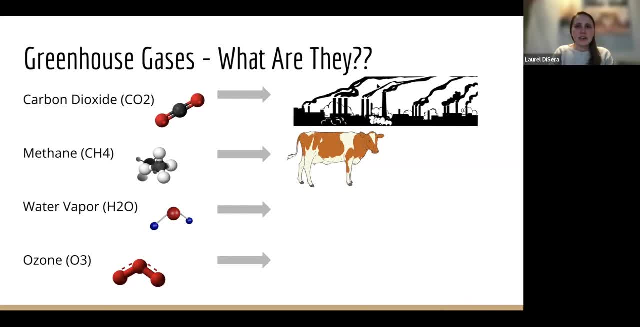 I know I know there are other initiatives happening in other places, but it seems like it's a really interesting tool that people are using and hopefully can implement more widely. So methane is actually more potent of a greenhouse that gas than carbon dioxide, So it's much worse. 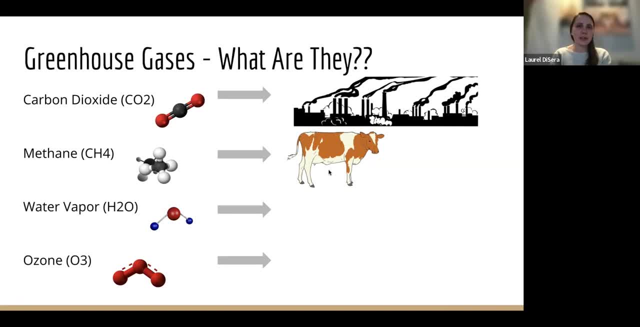 in the atmosphere, much worse for harboring heat. However, it is much less abundant, which we're really lucky for. If there was a lot more of it, we would be in really big trouble. The third greenhouse gas is water vapor, which I'm sure you're all familiar with When you heat. 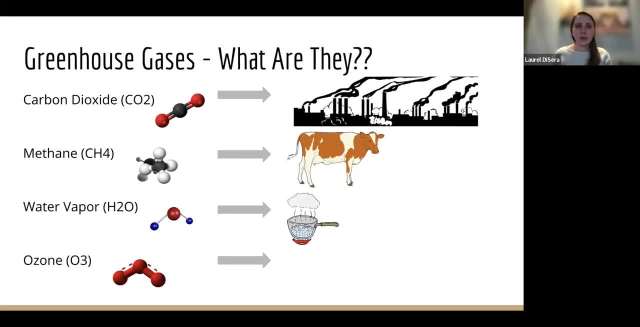 up water on the stove, you're going to have boiling water, which then releases water into the atmosphere, And you might do this to add humidity to your house when it's really dry, and so you're not constantly drinking water or having really dry skin. But water vapor is present in our atmosphere and it has been there since the. 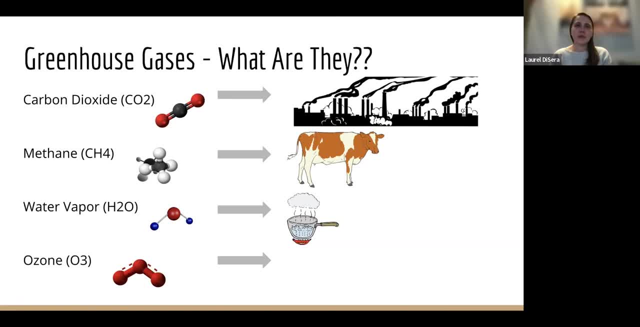 beginning of Earth, And water vapor is really important at maintaining Earth's habitability and keeping us warm within the greenhouse effect of how it was before we altered it with carbon dioxide, And I'm sure you all have heard and talked about the water cycle, which you know. 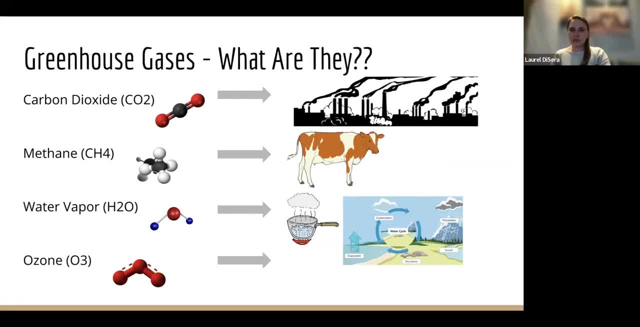 we have this evaporation forming into clouds and then rain, So water vapor is like a crucial part of the water cycle and also something that contributes greatly to our well-being and staying warm here on Earth. And then finally, ozone. Really don't get involved with ozone. Ozone is very dangerous. 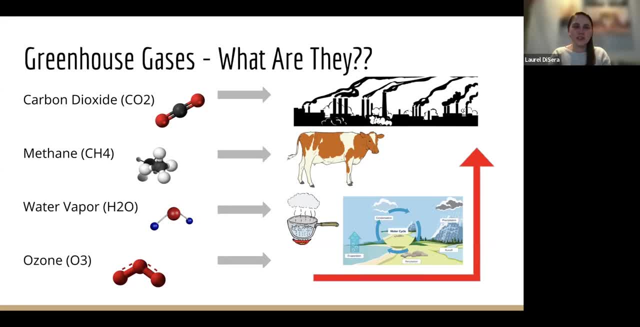 for you. if you're ever in a region where they're like high ozone levels, you need to get out of there. But ozone is essentially created through a chemical process in the atmosphere, when we have a release of carbon dioxide, for example, In regions that have carbon dioxide. 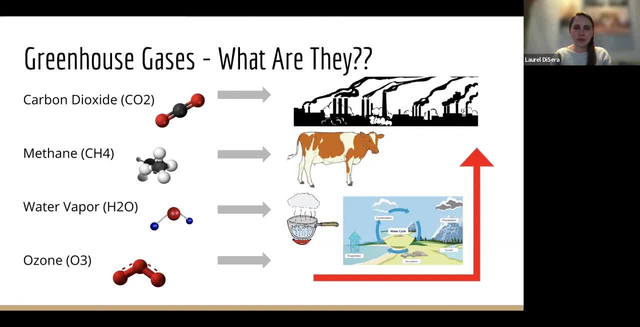 there are little atmospheric reactions that happen and ozone can be created. So these are kind of the four most important things that we need to be aware of when we're talking about erosion곱 Greenhouse gases. There are many others, but they have a lot smaller concentration in the 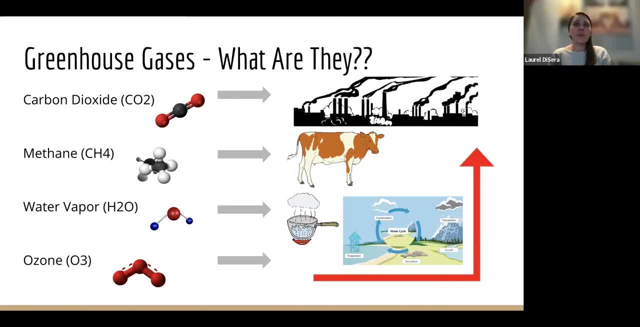 atmosphere and are a lot. They might be very potent, but they're. they just are a lot fewer and far between. when you look at all of the atmosphere, all the molecules in the atmosphere, There are other molecules that are. these are specifically greenhouse gases. But you have. 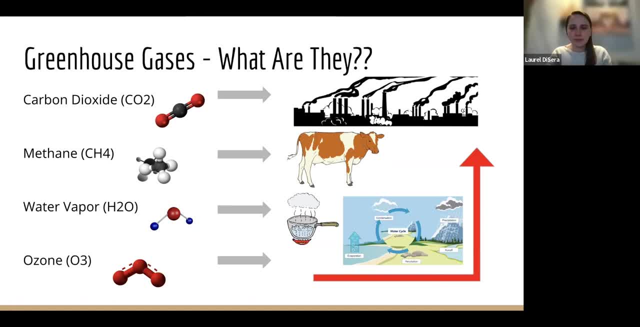 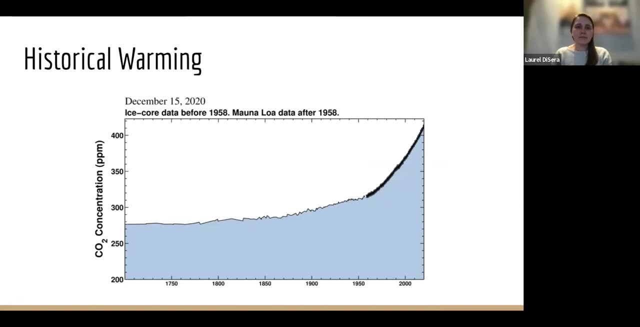 nitrogen and other molecules floating around too, And greenhouse gases, as I mentioned before, are kind of are doing. We are putting them into the atmosphere and we are really impacting temperature. So here is just our plot. that is, looking at carbon dioxide concentration that we see here on the y-axis And on the x-axis we see time. 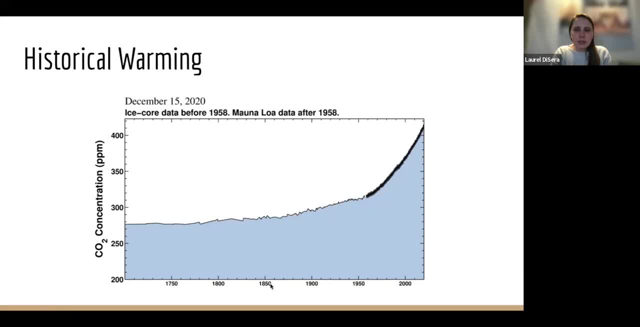 So it starts around 1700 and we see carbon dioxide concentrations increasing, but more so, increasing most rapidly after 1960. If you think about, maybe, why we started increasing in 1850, maybe the industrial revolution rings a bell and you can say, okay, maybe that's when we started. 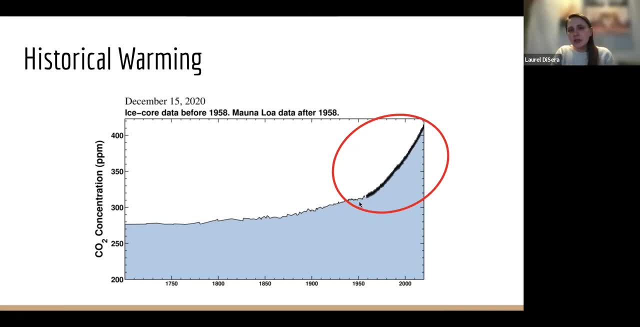 emitting. but you can see there's a pretty slow increase. And then all of a sudden- after 1960, we see this massive uptake in release of carbon dioxide. And this has to do with a variety of reasons which we can discuss. 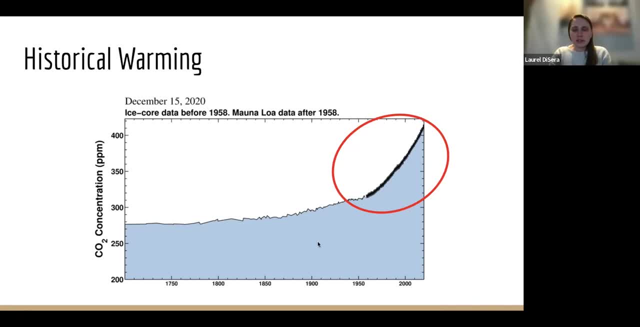 We can discuss that further length later if you're interested, But we've been tracking this information for a long time. This kind of darker part has been monitored at Moanalua, their big observatory on the big island of Hawaii. But before they were using ice core data which, if you, 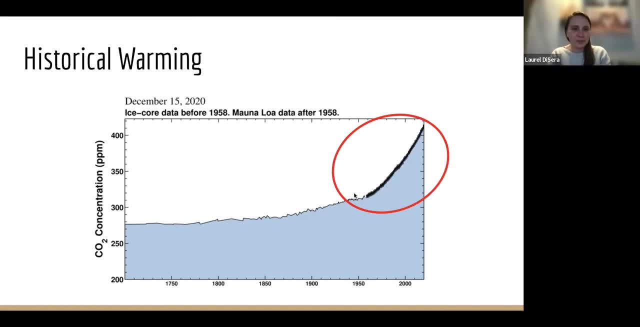 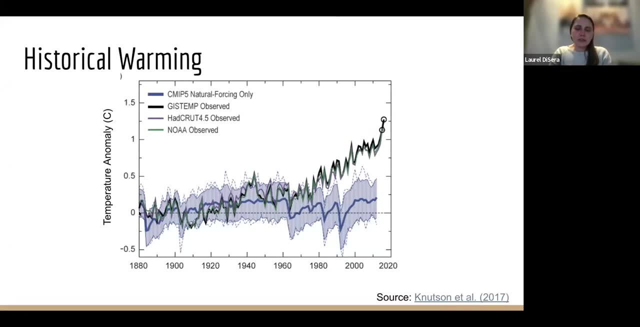 have questions I can also discuss about afterwards, because I scores are really cool And if we look at that here, we can see that since 1880, so this was a little bit shorter of a time. but if we look where we started to see an increase in the last plot in 1960, we can see this increase. 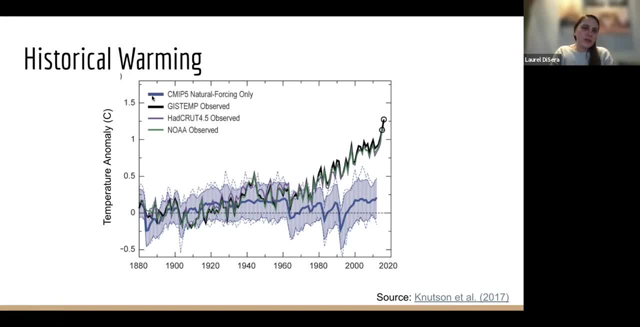 as well. This is looking at just temperature from a variety of different temperature monitoring devices or models, and this is looking at temperature anomaly again. So if we were to remove the average temperature, the annual average temperature, we would be left with some sort of 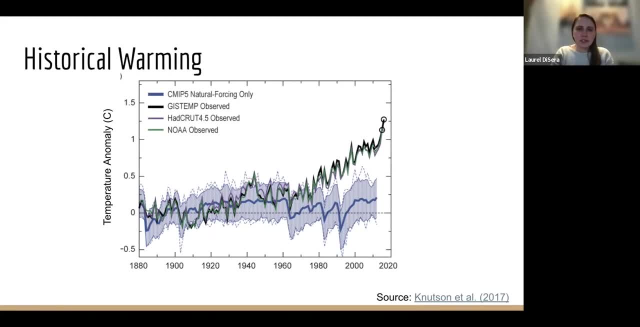 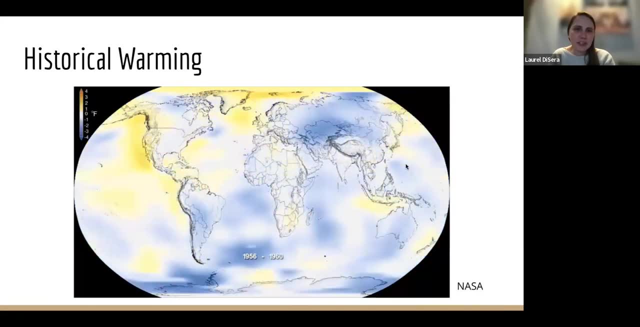 leftover, and we see that this leftover has been increasing pretty rapidly since 2020.. And we can see this visualized here as we get warmer and warmer and warmer, which actually is quite terrifying. You can see that the Arctic is warming very rapidly compared to many parts of the world, but it is very impactful. 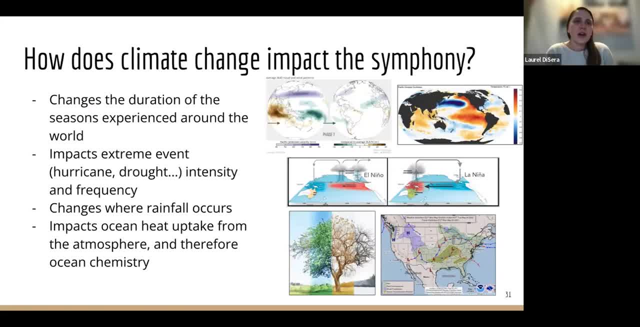 So the question comes to: how does climate change impact our climate symphony? Well, climate change- if you want to think of it in like the musical sense, and if you're not familiar with this term, that's okay, but you could think of the climate symphony. 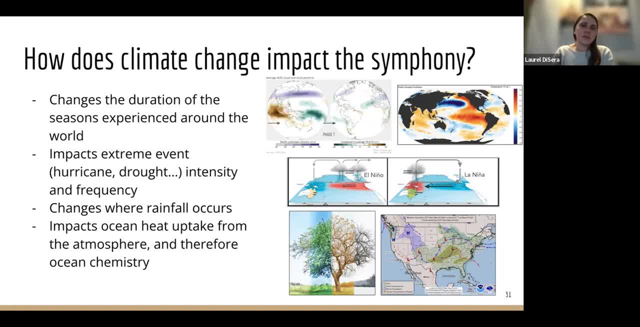 being modulated by climate change to another key, for example, or impacting how fast the tempo is of the music. How quickly are we changing our seasons? for example, The spring came awfully fast in New York this year and that might have to do with some climate. 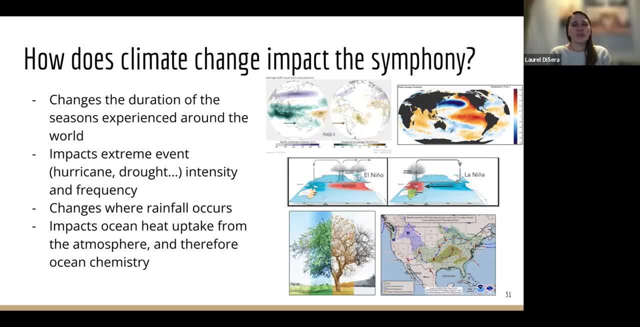 variability, but it also might have to do with climate change and I'm sure there are many scientists working to try to publish that information right now as we speak. But this can also impact extreme drought. It can impact hurricanes and intensity and frequency of hurricanes. It can impact where our rainfall is going to be changing. 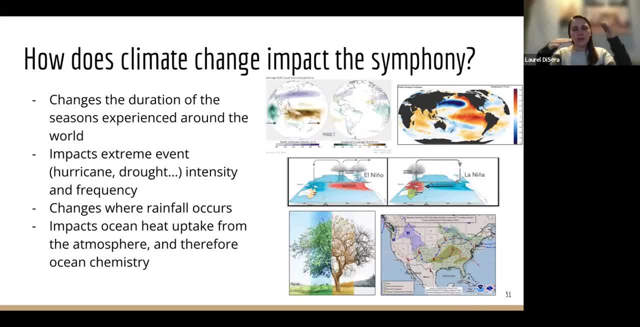 you know how we're going to be changing our rainfall around the equator, and if more places are going to be getting more rainfall than others and some places might be experiencing a drying overall, And then all of this has interface with the ocean, right? So as we get, 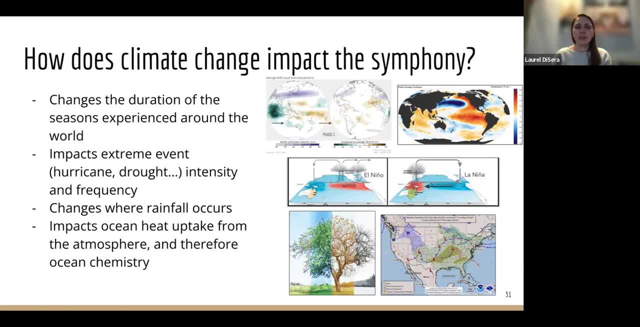 warmer and warmer. the ocean is going to have to take up some of our heat and this might take might impact how some of our longer scale climate variability or our climate symphony members behave. How are sea surface temperatures going to impact El Nino, or how are they going to? 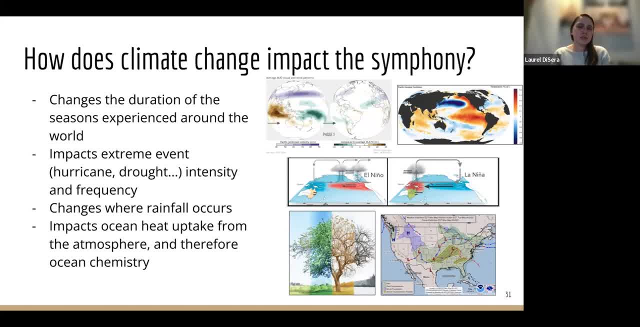 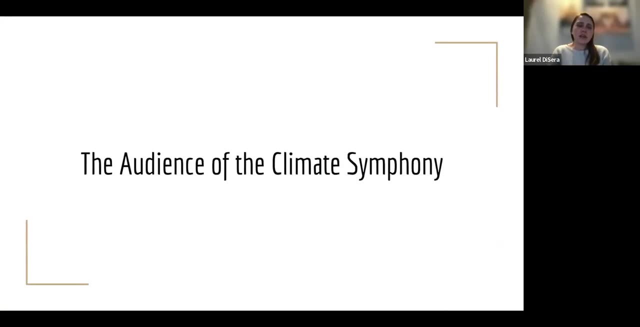 impact, the Pacific decadal oscillation And these are some questions we're still working on today to try to understand. But you know, all of this is interesting in the climate sense, but really we want to think about the audience of the climate symphony. Who's being impacted by our climate? 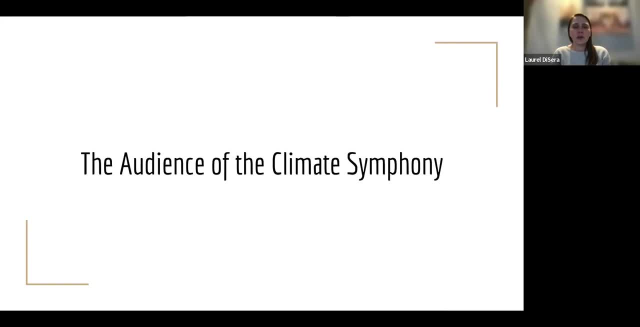 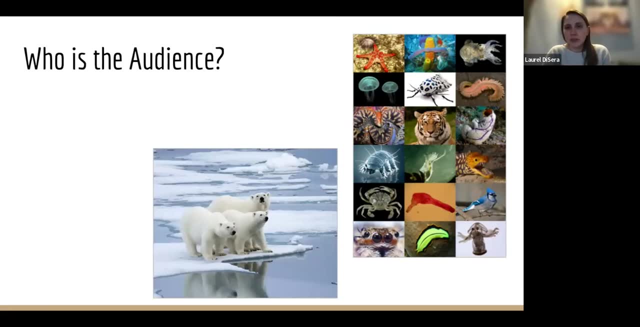 symphony. How is this changing the way that we live our lives, right? So I mean, first and foremost, before any humans get mentioned, there's a very diverse animal population, species of all different kinds that are being impacted by climate change, ranging from polar. 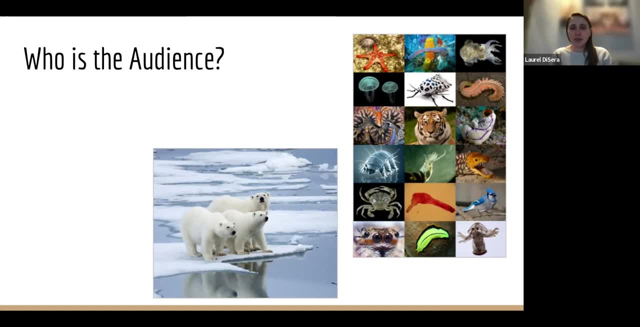 bears to aquatic species that I've never heard of in my life. But people are studying with great interest to try to understand how ocean communities and different forms of biodiversity and life are being impacted by climate change. But on top of all this climate change also impacts us and people's all kinds of jobs. 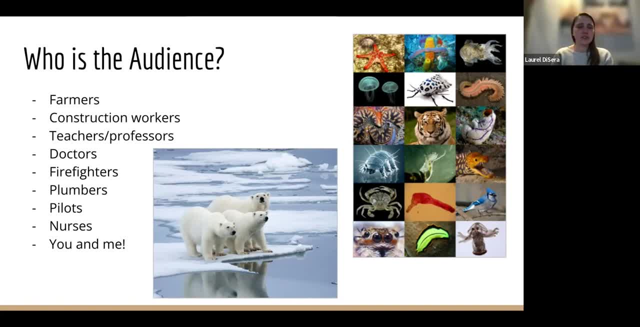 Farmers obviously are going to be impacted in the fields, as well as construction workers. teachers and professors are going to be impacted: firefighters for fires, for example, forest fires, or wildfires. pilots, depending on how the atmosphere responds to climate change, this might impact aviation. 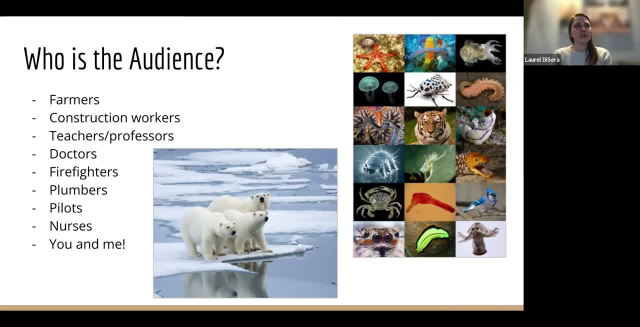 Nurses and surgeons. even I was talking to someone recently, that is, a surgeon, who was saying that transport of surgical equipment is being impacted by climate change because of the fact that, for example, extreme heat or extreme rain is impacting ability for the transport or the supply chain of goods, which I thought was really interesting. 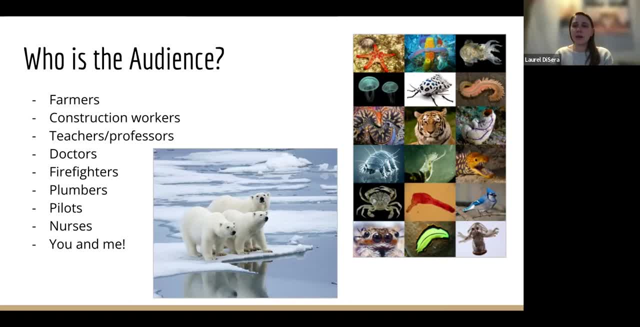 and something that, like I, had not even thought of and that's impacting how many surgeries can be done or the quality of surgery. So this is going to impact everyone and it is impacting people as it is, And so we are all the audience of the climate symphony and how it is changing. 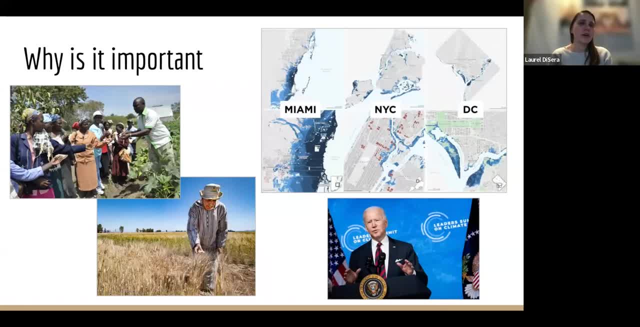 And this is important for a variety of reasons, like I mentioned before, whether that be for farming in the United States or anywhere in the world, but also for flooding and flood risk from hurricanes or sea level rise, And this is something that our leaders have been. 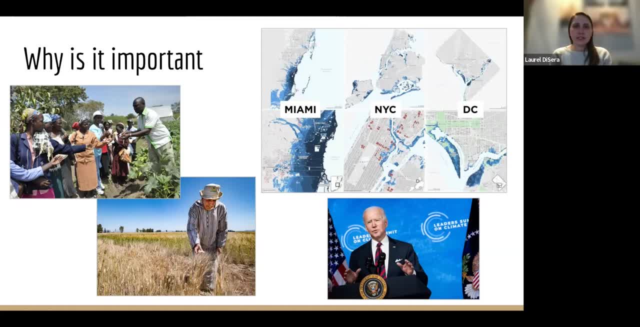 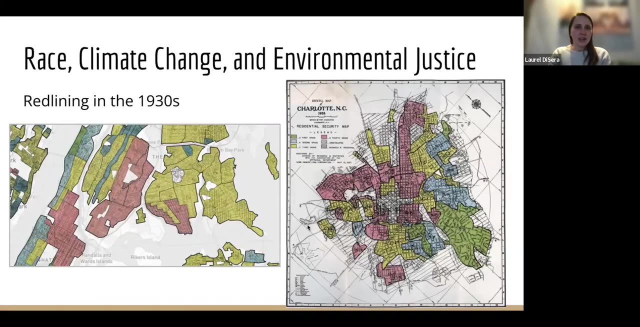 working on for a long time, More recently with recent infrastructure and legislation that has been passed. So that's, I mean, at least pretty encouraging from the US perspective as of late. But I also wanted to mention how this is also impacting the people of different communities. 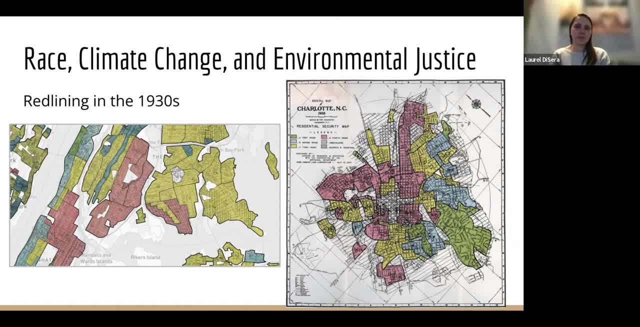 based on previous policies that have been made in the United States, for example, and how it's impacting folks of different races- And I feel like this is- I almost see this daily in the news- and how redlining, for example, or other forms of segregation that have. 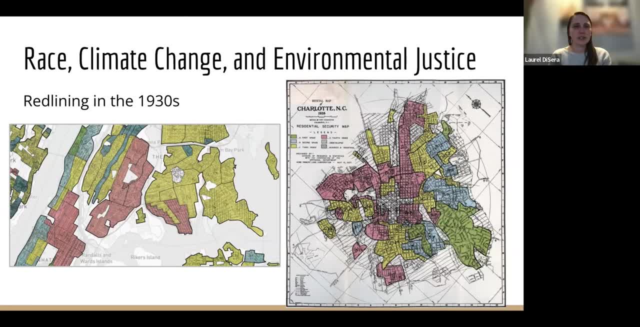 happened in the 1930s or before are impacting people differently. So redlining just as a brief introduction. if you have questions, we're almost at the end and I can explain more. But redlining was essentially done in the United States in many large cities in the 1930s. 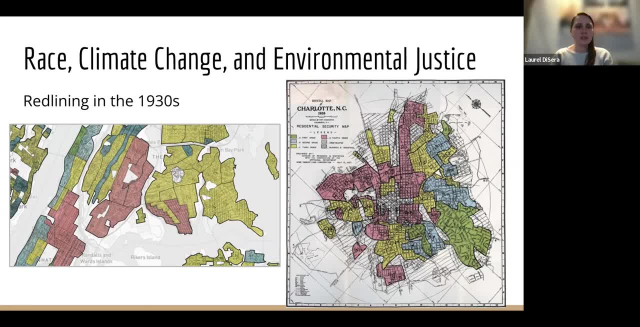 and effectively pushed communities of color, specifically Black communities, in particular neighborhoods and gave their property values lower values and primarily white neighborhoods, And a lot of these communities that are redlined or red-colored, as you can see here, have struggled with environmental-related concerns. They have been 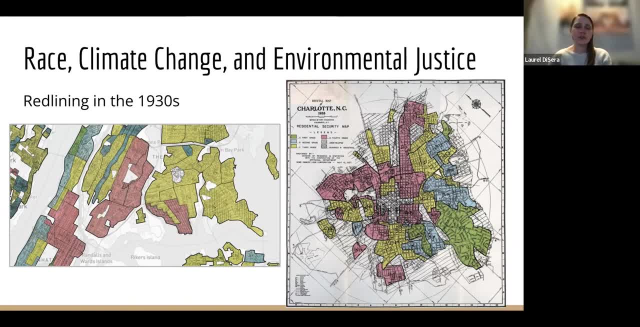 exposed more severely to pollution, and unjustly. I feel like I'm on The Guardian every day, reading different things that people are coming and studying and finding that have been impacted by redlining in the history of the United States. So this is something that researchers are working. 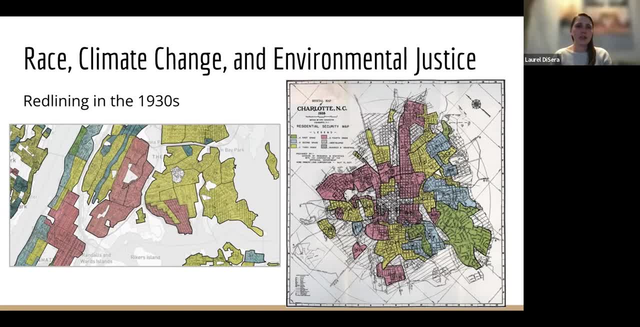 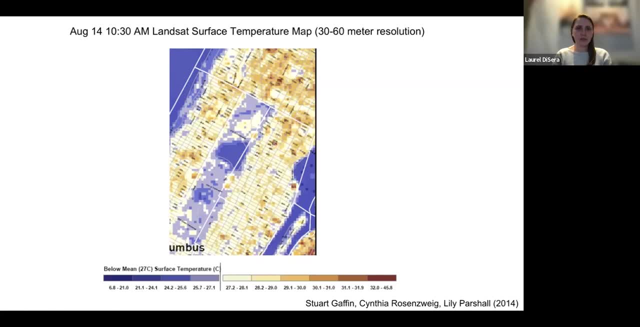 on trying to understand how to be more environmentally and climate just when it comes to actions that we're moving forward, And one example in the Harlem area that you may know or understand is: this is a picture of New York City looking at surface temperature And we can see that the cooler areas are blue here and the warmer areas 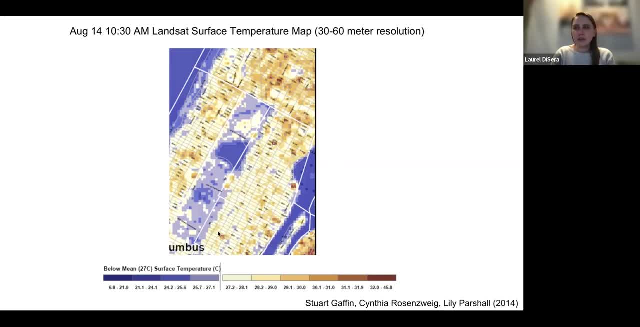 are red, And when you're on the east side, for example, you can see that it's maybe not too cool or not too warm, But if you move up into Harlem it gets much warmer, And so understanding how we can study and implement climate change adaptation and mitigation in a way that's climate and 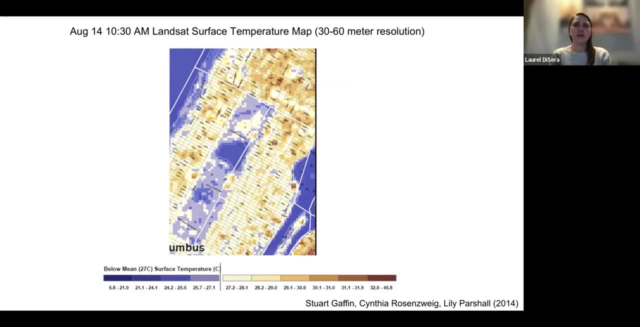 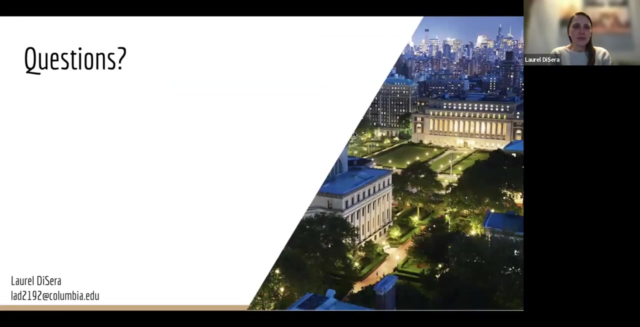 environmentally just is really important And really like harkens back for us to better understand how climate change is happening and how climate variability or our climate symphony is also changing and what that means for all of us and our future on this earth. So that's what I have today. I'm so glad that you were able. 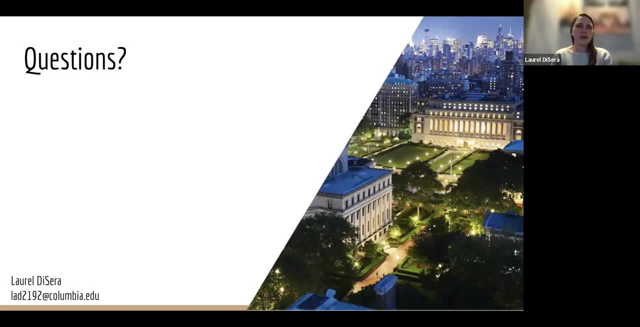